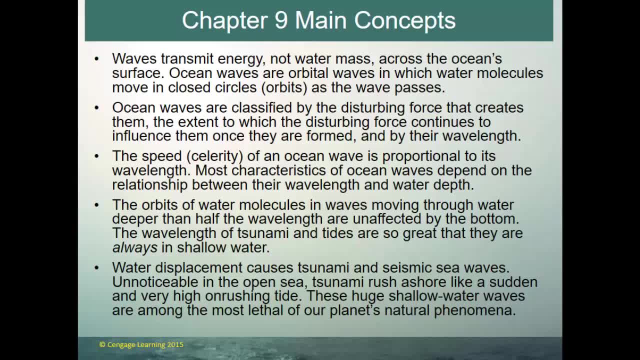 waves, And most characteristics of ocean waves depend on the relationship between their wavelength and the depth of the water in which they're traveling. The orbits of water molecules and waves moving across the ocean are called waves And the orbits of water molecules and waves moving 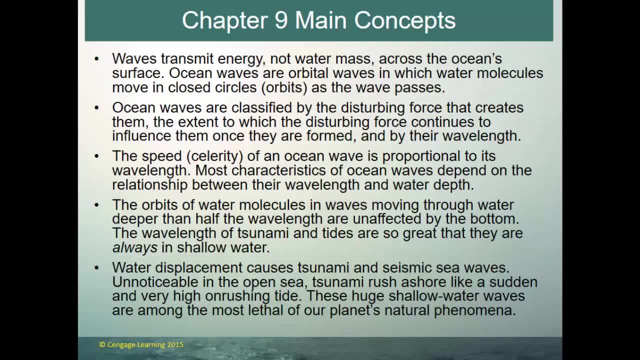 through water deeper than half the wavelength are unaffected by the bottom. That means in deep water waves can be unaffected by the bottom. The wavelength of a tsunami and tides are so great that they're always affected by the bottom, So they're always considered to be in shallow water. 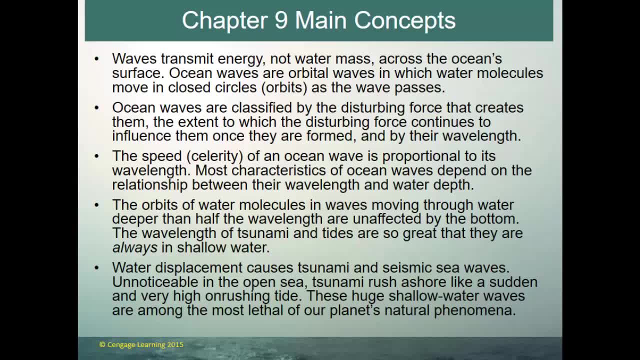 And water displacement causes tsunamis and seismic sea waves. That's going to be very important when we talk about earthquakes and what creates tsunamis. Tsunamis are literally not noticeable in the ocean, but they rush ashore And they're not noticeable in the ocean. 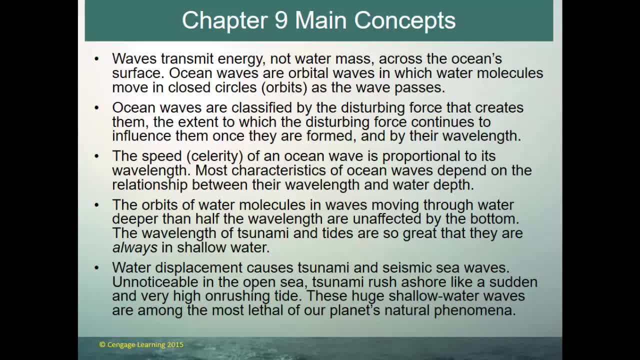 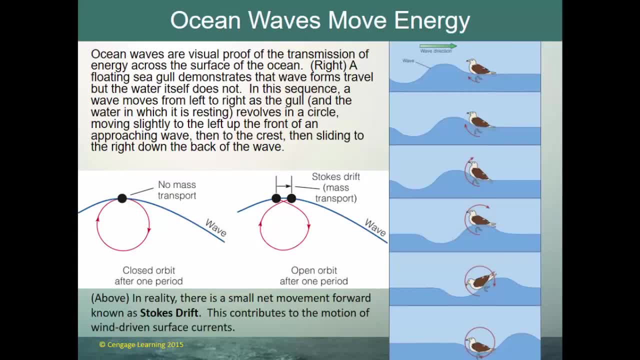 but they have a very high on-rushing tide. They are huge shallow water waves and are among the most lethal of our planet's natural phenomena. All right, ocean waves move energy. Ocean waves do not move water, They move energy. Ocean waves are visual proof of the transmission of energy. 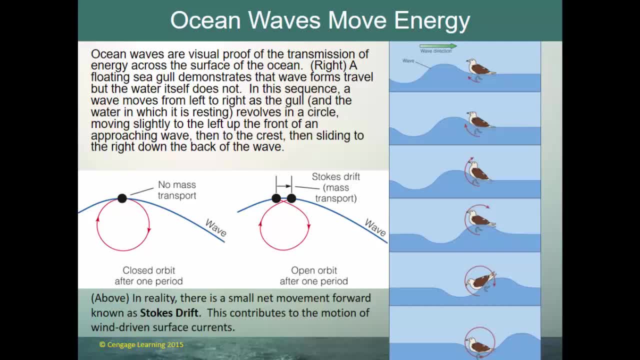 across the surface of the ocean. To the right we can see a floating seagull and it demonstrates the way a wave travels the ocean and passes through the ocean, And it's actually a very powerful wave. But the ocean is still moving. It's moving at an incredible speed And it's moving at a magnetic. 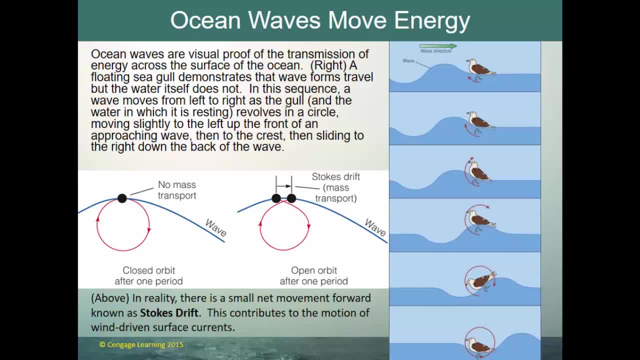 rate. So it's moving at a highly electric rate, So it's moving at an international velocity, So travels, but the water does not. You can see, the wave moves from left to right and the gull and the water in which it's resting revolve literally in the circle. 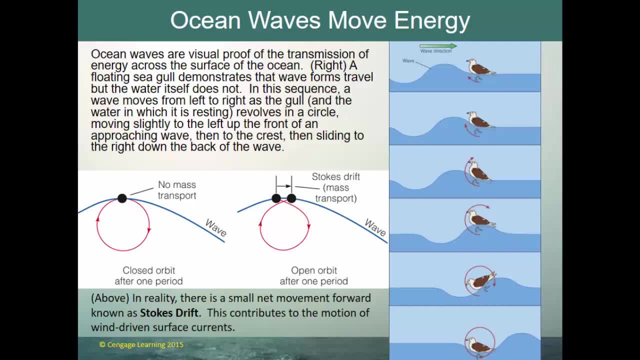 moving slightly to the left up the front of the approaching wave, then to the crust and then sliding to the right down the back of the wave, And we can see how that works in this illustration below. There's no mass transport of the well. there's no mass transport, nothing moves. the water doesn't move, the energy moves. 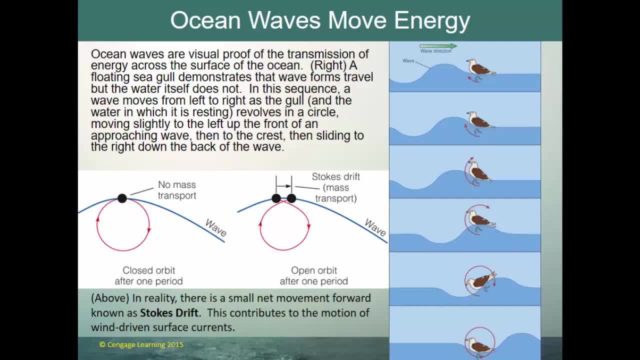 through the water And so in the actual wave there is this very small amount of movement which is known as Stokes drift, and that is the the amount of transport that actually happens in an actual ocean wave. So in reality there's a small net movement forward and that's known as Stokes drift, and this contributes to the 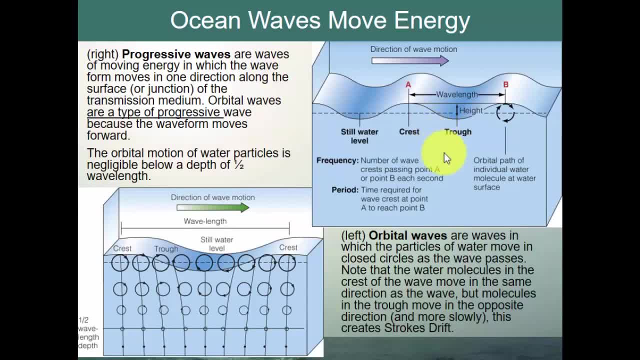 motion of wind-driven surface currents. The height then is between the top of the crust and the base of the trough. That's going to be the height Now. the frequency is the number of wave crests: crest 1, crest 2, passing point A or B each second. So for every crest that, 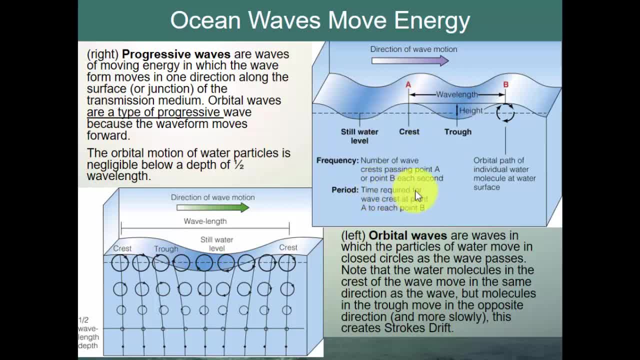 passes by per second. that's the frequency. The period is the time required for a wave crest at point A here to reach point B, And again, this is the orbital path of the individual water molecule underwater. So orbital waves are waves in which the particles of water move in closed circles as the water. 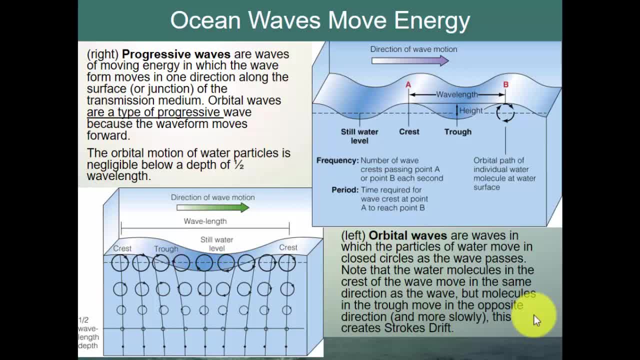 passes. Note that the water molecules and the crest of the wave move in the same direction as the wave. The molecules in the trough move in the opposite direction, but they also move more slowly, and the reason and the fact that they move more slowly is why you have that orbital drift or that Stokes drift. How do we? 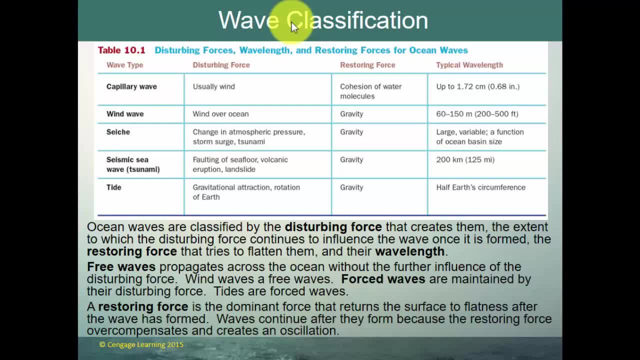 classify waves. Scientists always want to classify natural phenomenon, so we're going to classify waves. We have the wave type, the disturbing force, the restoring force and then the typical wavelength. So we're going to classify the wave type as capillary waves, wind waves, sea. 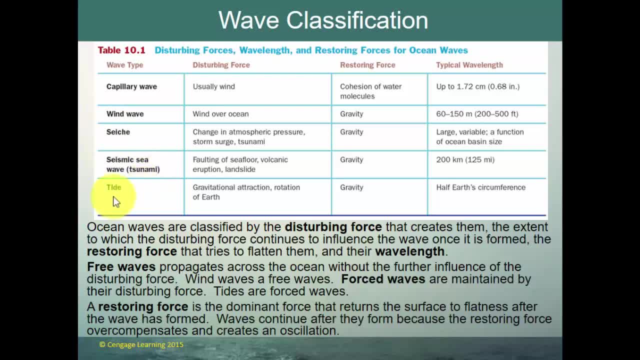 waves and then the typical wavelength. So we're going to classify the wave type as seismic sea waves or a tsunami or a tide, And the disturbing force of a capillary wave is wind. The disturbing force also of a wind wave is wind. A seiche is a. 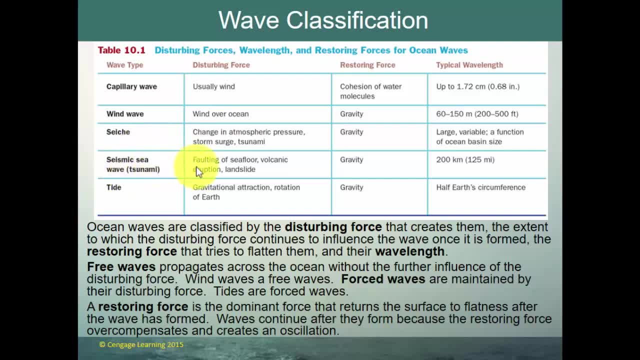 change in atmospheric pressure or which could also be storm surge, A seismic sea wave is faulting of the seafloor, a volcanic eruption or a landslide, And the disturbing force of all tides is the gravitational attraction of the Earth's Sun and its 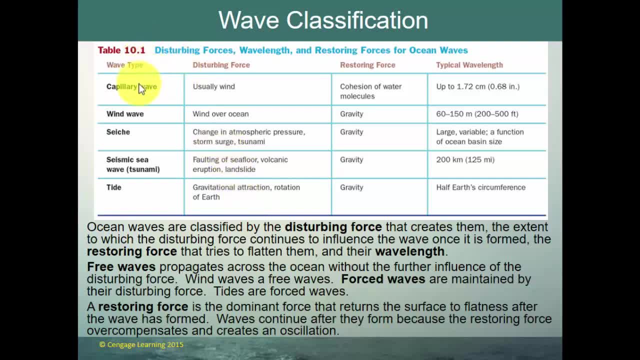 Moon and the rotation of the Earth. Now, what causes waves to? so? that's what disturbs waves, these issues. what causes waves to go back to where they were? Capillary waves, little, tiny waves. the cohesion of water molecules can actually bring them back down to flat. And all other waves, it's the restoring. 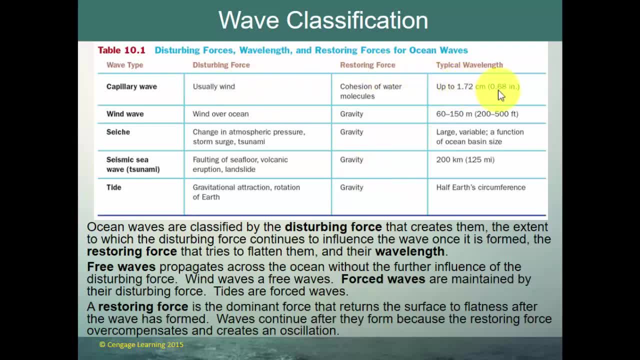 force is gravity. Now, the typical wavelength of capillary waves is just very, very small, just over half of an inch. The typical wavelength of a wind wave is anywhere between 200 and 500 feet, And then a seiche is going to be much larger and variable as a function of the 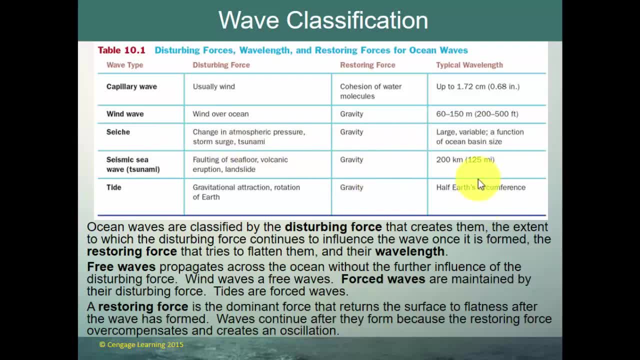 ocean basin, A seismic sea wave, you have a wavelength, and that means that the distance between crests of a tsunami could be as much as 125 miles, And then the wavelength of a tide is half the Earth's circumference. So ocean waves are classified by the disturbing force that creates them, The extent to which 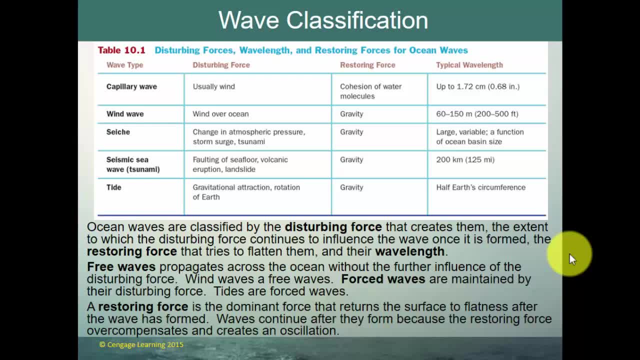 the disturbing force continues to influence the wave once it is formed and the restoring force to flatten them. So the disturbing force creates the wave and continues to influence the wave and the restoring force is the force that tries to flatten them. And the third way that they're 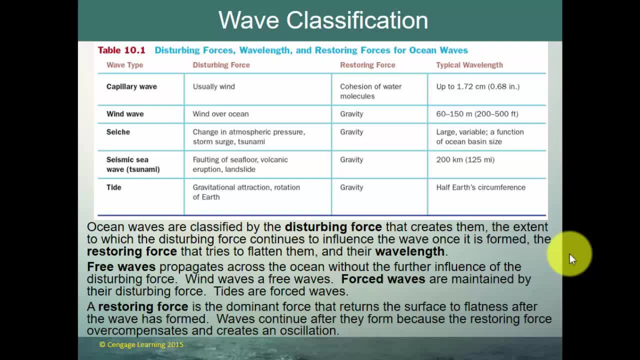 going to be classified is by wavelength. Free waves propagate across the ocean without further influence of the disturbing force. So a free wave is going to be disturbed by wind and then continue to move across the ocean and most wind waves are free waves. Force waves are maintained. 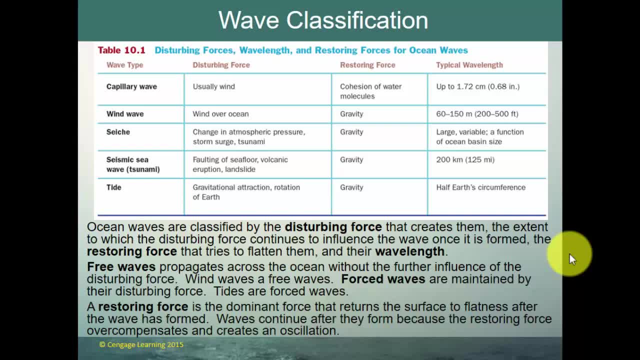 by the disturbing force. so tides are considered to be forced waves And a restoring force is the dominant force that returns the surface to flatness after the wave is formed. Waves continue after they form because the restoring force overcompensates and creates an oscillation. So a wave once. 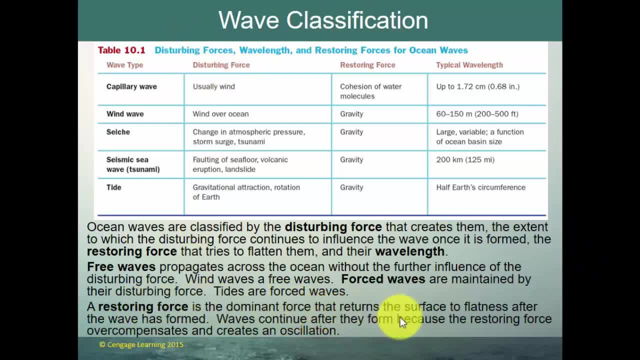 it leaves, its disturbing force continues because the restoring force tends to create overcompensation, meaning it may pull the wave down to the surface level, but it also pulls it below the surface level, which is the force created by the wave, And it creates an oscillation which is called the pinched net force. 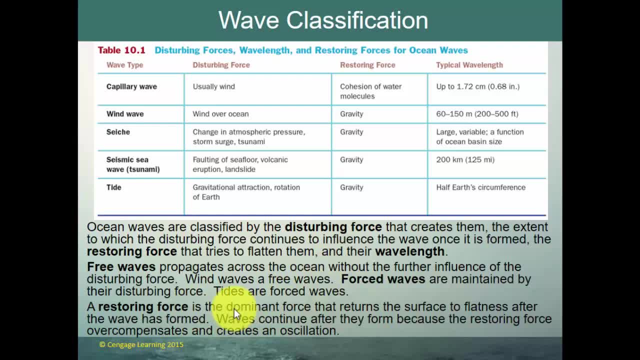 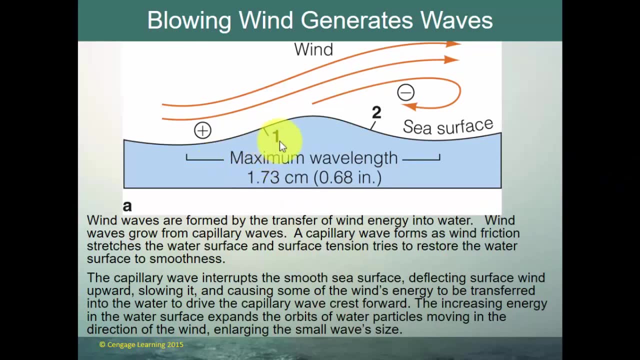 and so it responds by going up above the surface level. so waves that continue after they form free waves do so because the restoring force over compensates and creates an oscillation. all right, so this is how your typical wind wave, and so this is going to be a capillary wave, very, very small wind. 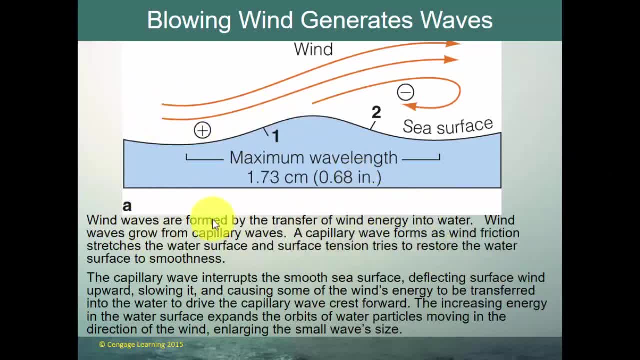 waves are formed by the transfer of wind energy into the water. wind waves grow from capillary waves, so all wind waves start as capillary wave. capillary wave forms as wind friction. literally the friction between the wind and the surface of the water stretches the water and the surface tension tries to restore. 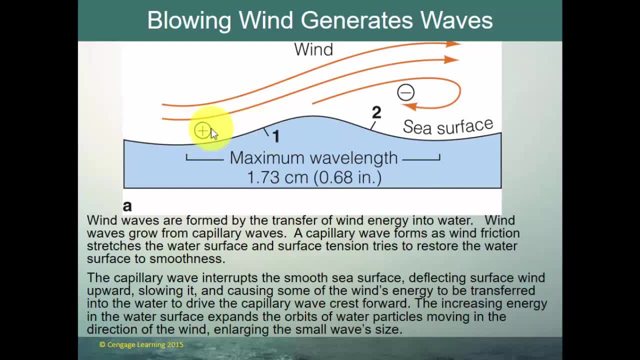 the water to smoothness. so the wind stretches the water out and surface tension tries to pull it back. the capillary wave interrupts the smooth sea surface, deflecting surface wind upward, slowing it and causing some of the wind energy to be transferred into the water to drive the capillary 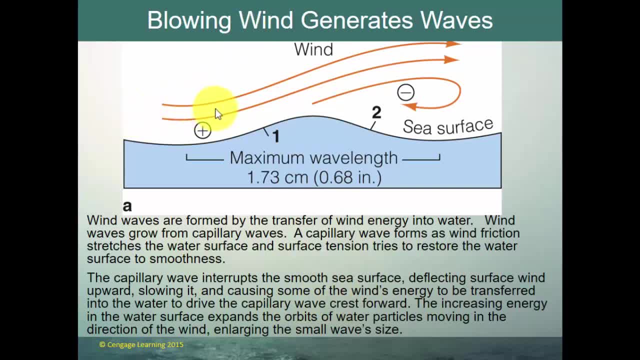 wave crests forward. essentially, the wave flows across flat water stretches. it pulls it up and creates a spray, tiny capillary wave. the increasing energy in the water surface expands the orbital of orbits of water particles moving in the direction of the wind and enlarges the way of size. so once the capillary wave 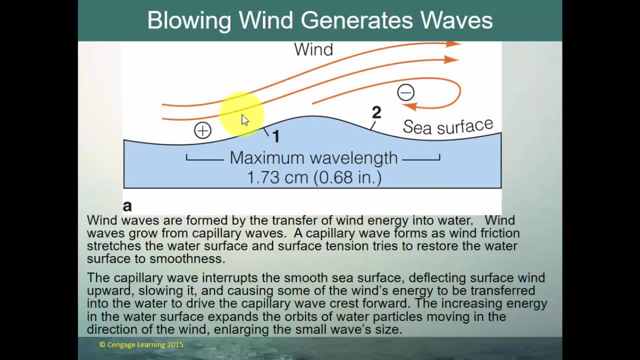 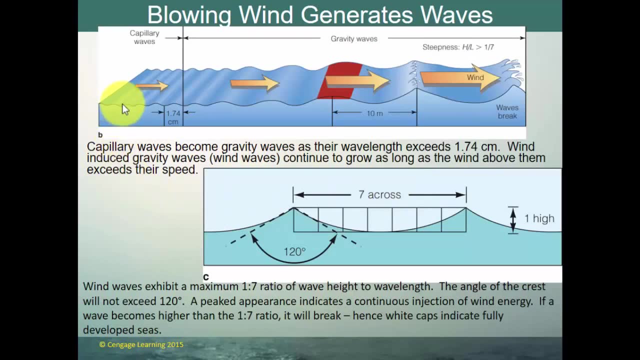 is formed. this tiny wave- continued wind blowing the back of the capillary wave, expands the orbits of the water bottle particles moving in the direction of the wind and enlarges the wave size. So this is what it looks like, with capillary waves with the wind stretching the water. the 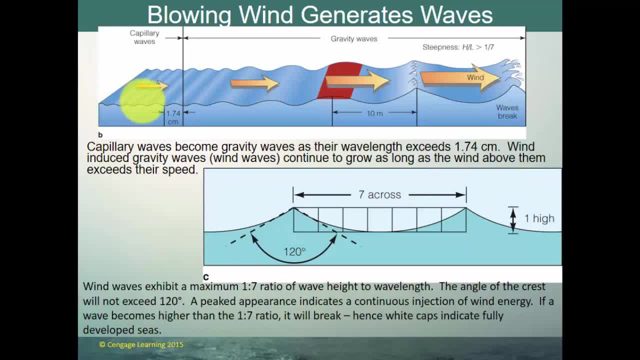 surface cohesion of the wave of the water that is trying to pull it back to flatness and you get into capillary waves. Continued wind blowing in the back of the capillary waves causes those waves to continue and eventually the restoring force, gravity- pulls the water down below the surface. then it comes. 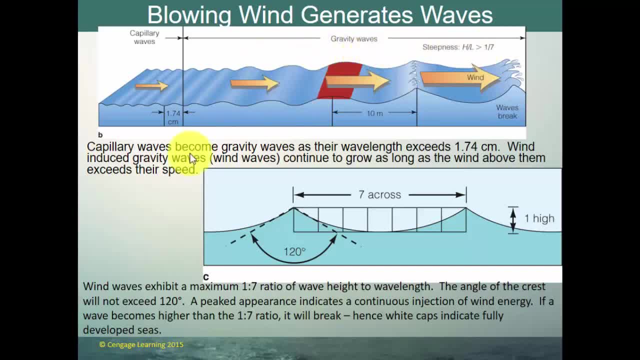 back up and you get the free wave that that continues. So capillary waves become gravity waves as their wavelength exceeds 1.74 centimeters. so once it gets above 1.74 centimeters, then you have these gravity waves. these, these free waves, Wind induced gravity waves or wind waves continue to grow as long as the 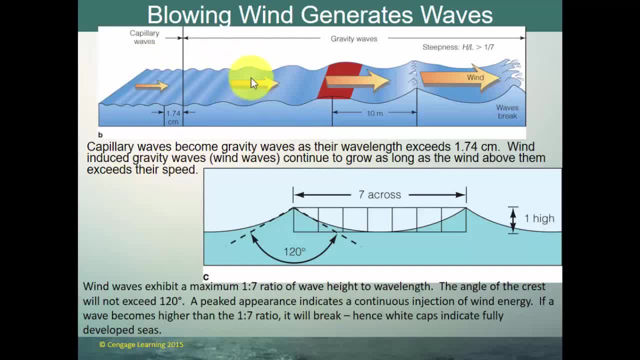 wind above them exceeds their speed. So if the wind is blowing faster than the speed of the wave, the wave will continue to get bigger. Now wind waves will exhibit a maximum 1 to 7 ratio of wave height to wavelength. so this is the wave height from the trough to the crust. this is the wavelength from one trough. 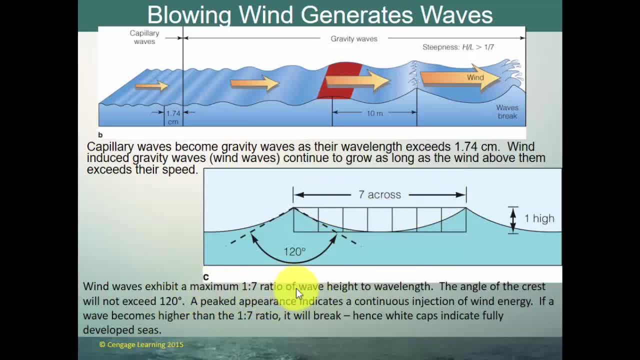 to the other. wind waves exhibit a maximum 1 to 7 ratio. the angle of the crust will not exceed this 120 degree angle. a peaked appearance indicates a continuous injection of wind energy. if a wave becomes higher than the 1 to 7 ratio, it will break, and that's where we get white caps. so winds will look like. 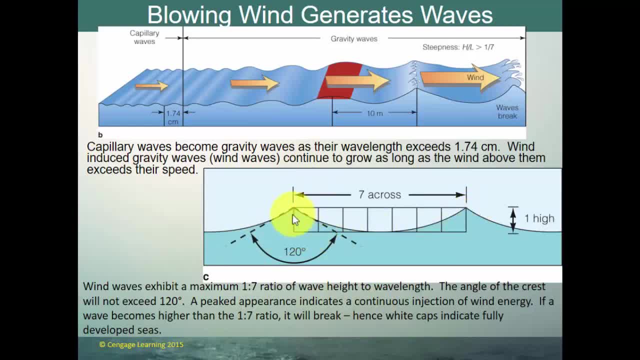 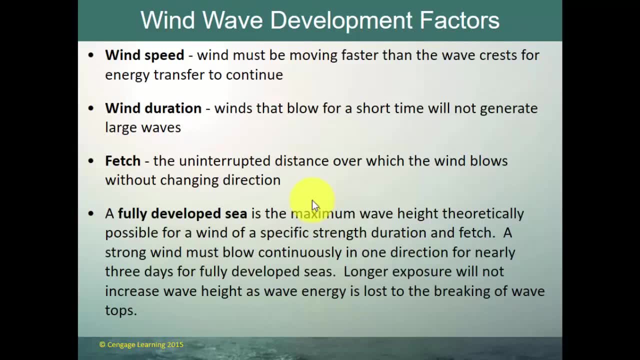 these peaks in the water until you get to this greater than 1 to 7 ratio, and then you'll start to get white caps, and that occurs in what is known as fully developed seas. so wind speed: the wind must be moving faster than the wave crest for energy to energy transfer to continue. so these are the wave, or the 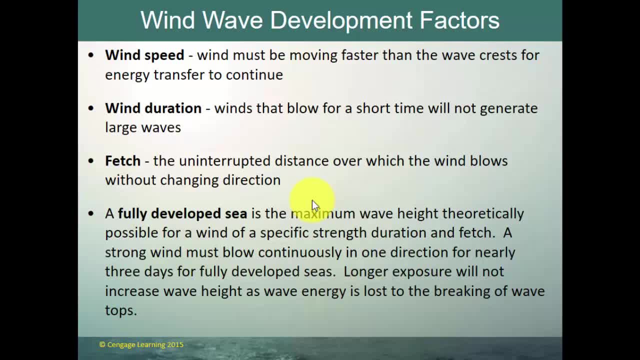 wind wave development factors. the wind speed must be moving faster than the wave for the energy transfer to the wind wave to continue wind duration: winds that blow for a short time will not generate large waves. winds that blow for a long time, however, will generate large waves. fetch is the uninterrupted distance over which the wind blows without changing. 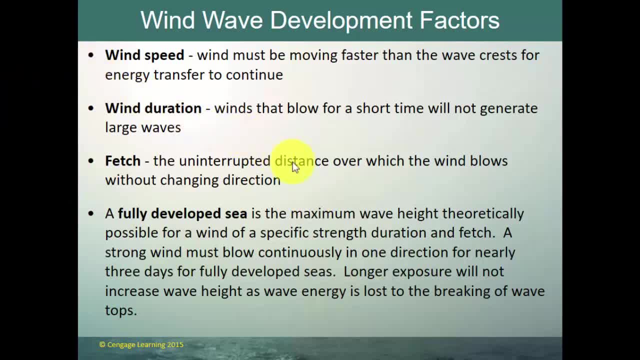 direction. so if the wind is blowing a straight line over a great distance, that's a long fetch of wind and that's more likely to develop larger waves. and so this concept of a fully developed sea is the maximum wave height theoretical possible for a wind at a specific strength, duration and fetch. a strong 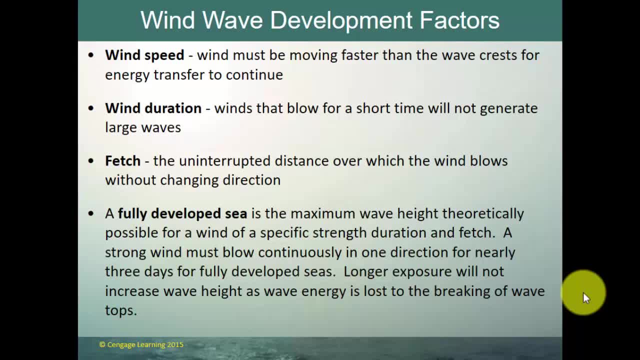 wind must blow continuously in one direction for nearly three days for fully developed seas to occur. longer exposure will not increase the wave height as the wave energy is lost to the breaking wave top. so this idea of fully developed seas: the biggest wind wave you can have from a type of wind is a. 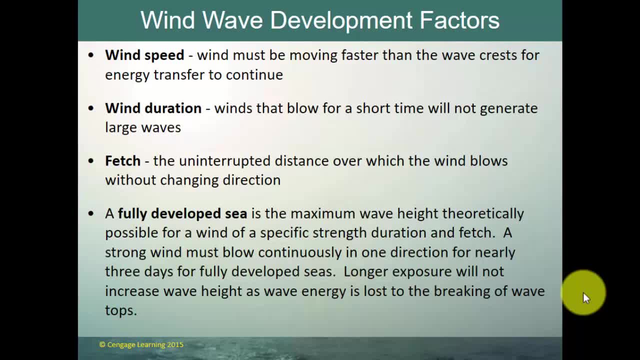 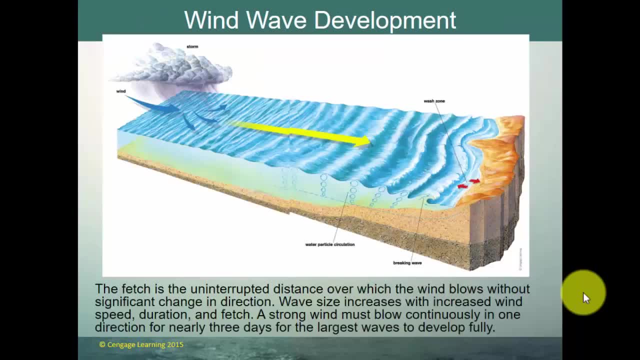 function again of the wind blowing across a specific stretch of ocean for a specific period of time. in a fully developed sea typically takes three days to form. So the fetch of the uninterrupted distance over which the wind blows without significant change in direction, the fetch is that uninterrupted distance. This is the fetch. 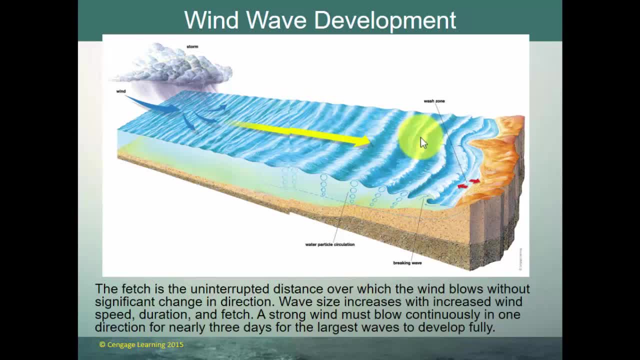 of the wave, from where the wind's blowing all the way to where it's no longer blowing. Wave size increases with increased wind speed. faster the wind, the larger the wave. increased duration of wind, the longer it blows and the fetch the length of distance that is that the wind blows over. 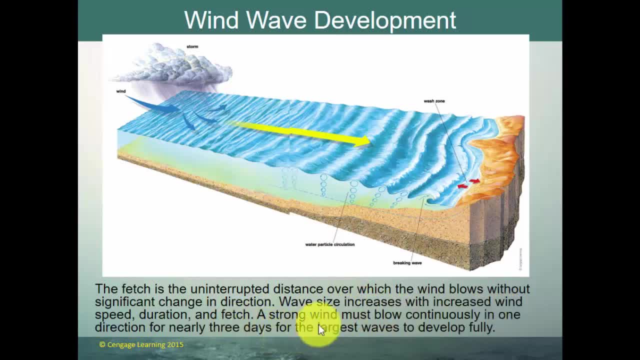 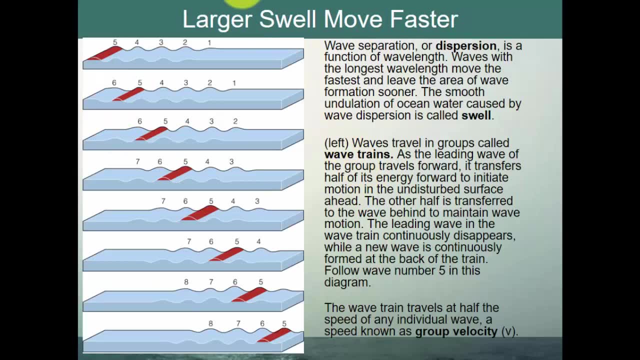 A strong wind must blow continuously in one direction for nearly three days for the largest wind waves to develop into the fully developed seas. All right, larger swell move faster, So this is going to be an interesting look at wave trains and how waves move through the open ocean. Wave separation or dispersion is a function. 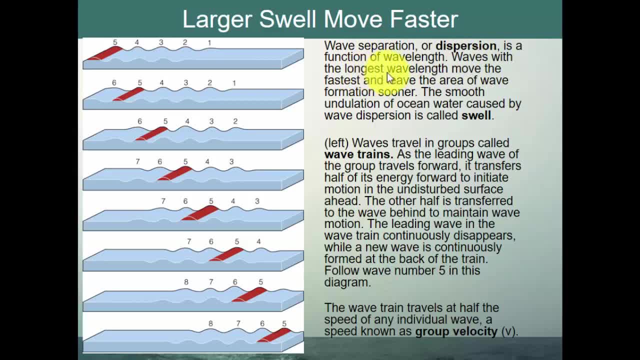 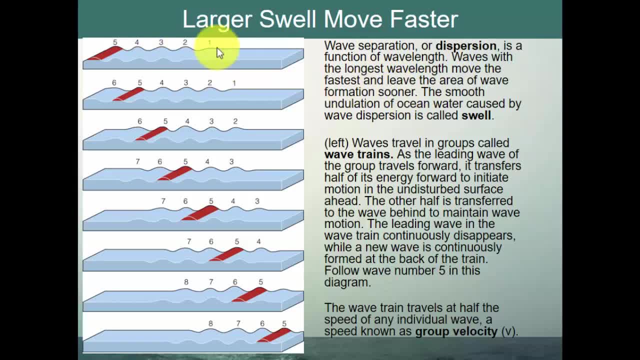 and leave the area of wave formation sooner, So longer wavelength waves will move away from the area of the disturbing force more quickly. The smooth undulation of ocean water caused by wave dispersion is called swell, So here at the left. waves travel in groups called wave trains, So one 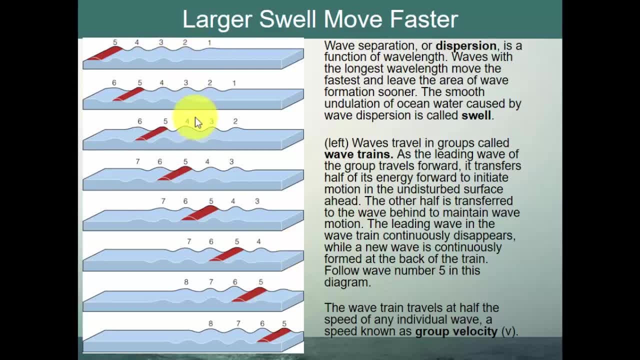 through five, one through six, one through seven, one through eight, one through nine, one through sixty, one through fifty, one through fifty. I'm torn. Pneudo- unwilling type of wave. then one becomes one. that's exactly the way waves behave. Pneudo wave seems natural. 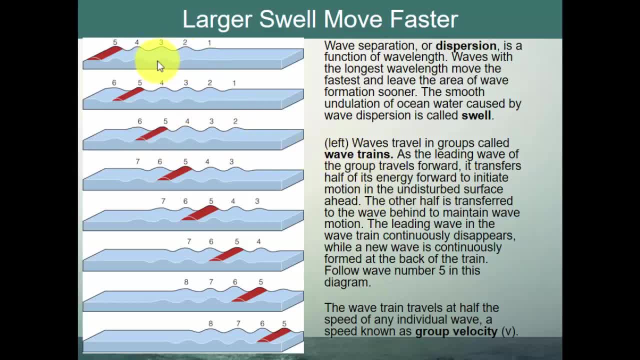 Okay, hazard, these are Egyptian ways. Yeah, basically, waves in a extremité either pass through the ocean or collapse, But Allied Starts and doesn't set aelandmovies. a permanent position in the ocean, going up two percent degrees. 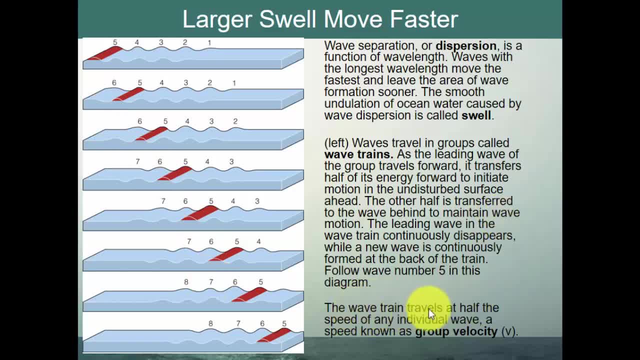 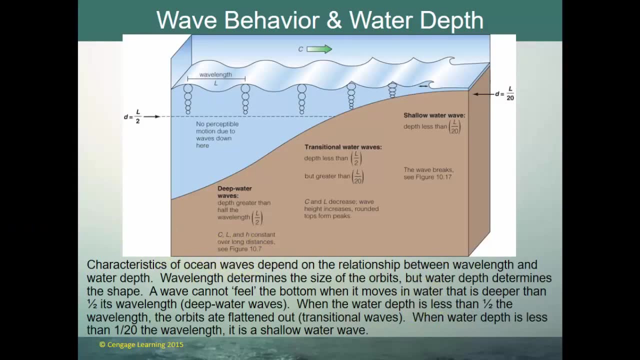 formed, and then seven is formed, and then eight is formed. The wave train travels at about half the speed of any individual wave, and so that speed of the wave train is known as group velocity. So how do waves behave in different water depth? Again, if you take the wavelength L and divide it, 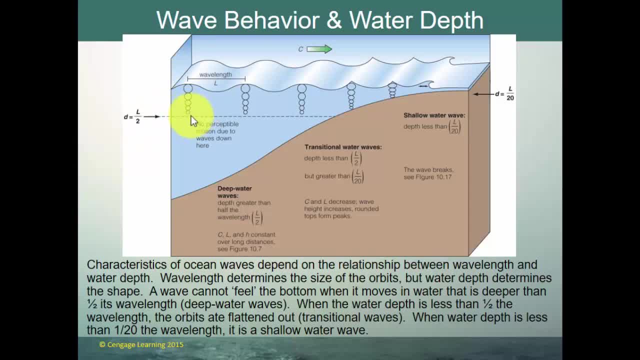 by two. that is the depth in which wave motion or orbital motion stops. So there's no perceptible motion underneath this depth. So as the wave moves into shallower and shallower water, you begin to lose that depth and it starts to impact the behavior of the wave. So ocean waves. 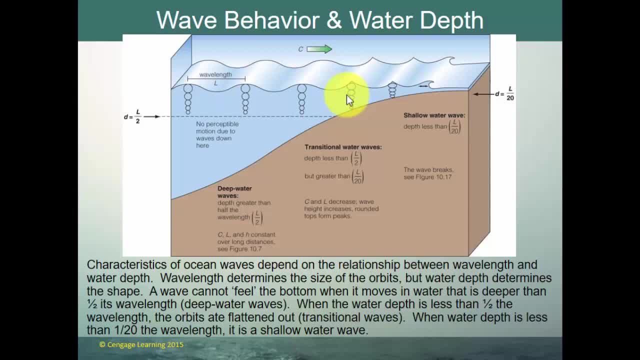 and how they act depends on the relationship between the wavelength and the water depth. Wavelength determines the size of the orbits, but water depth determines the shape. So how big these orbits are are a function of the shape of the wave. So if you take the wavelength L and divide it by two, 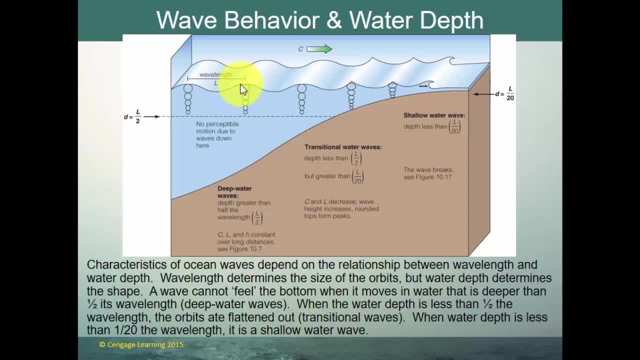 you get half of the wavelength, with a longer wavelength having much larger orbits. They are nearly circular in open water. but once they get into a depth that's half their wavelength those orbits begin to flatten out, So a wave cannot feel the bottom meaning these waves are. 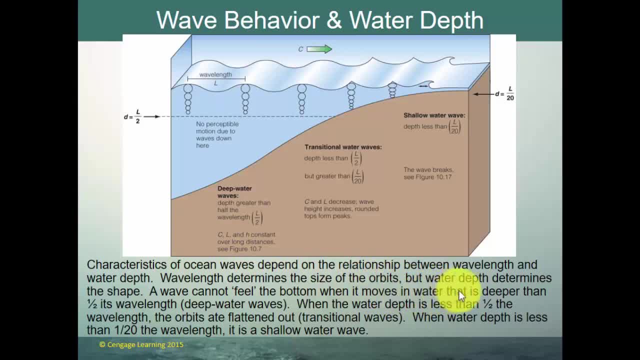 not feeling the bottom until the water is half the wavelength. So out here in the deeper water, they don't feel the bottom. Once they get into the shallower water, they begin to feel the bottom When the water depth is half the wavelength. they don't feel the bottom, So they don't feel the bottom. 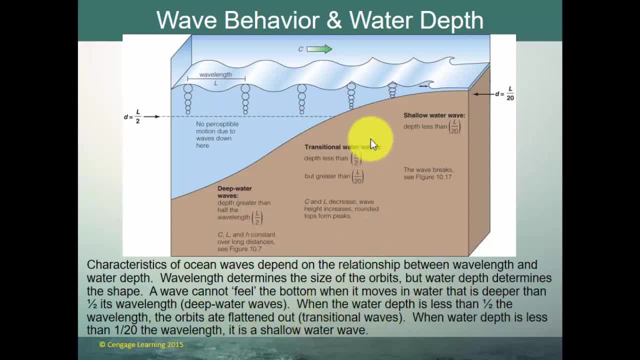 The orbits are flattened out and they become transitional waves. When the water is less than 1: 20th of the wavelength, it's considered a shallow water wave and that's typically where you start to see these breaking waves. In general, the longer the wavelength 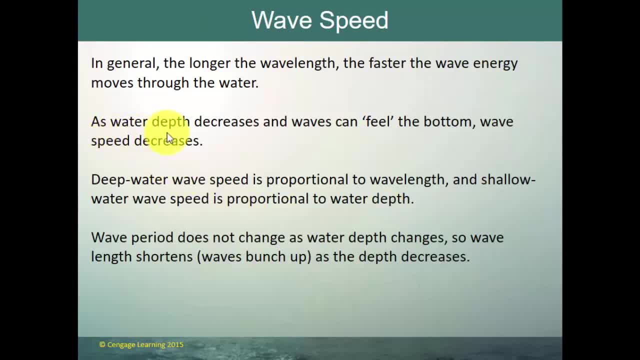 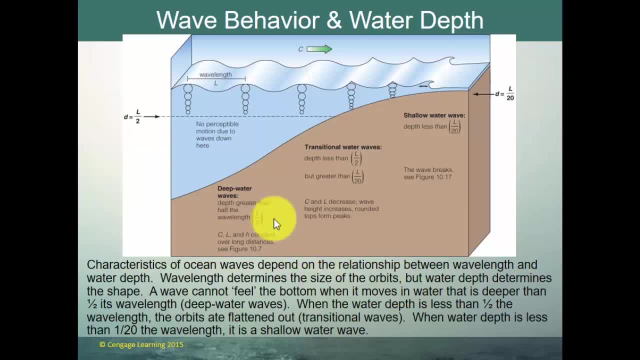 the faster the wave energy moves to the water. As water depth decreases, a wave can begin to feel the bottom and then the wave speed slows, And what ends up happening is because the wave speed slows as these waves move. the wave speed slows, So the wave speed slows and the wave speed. 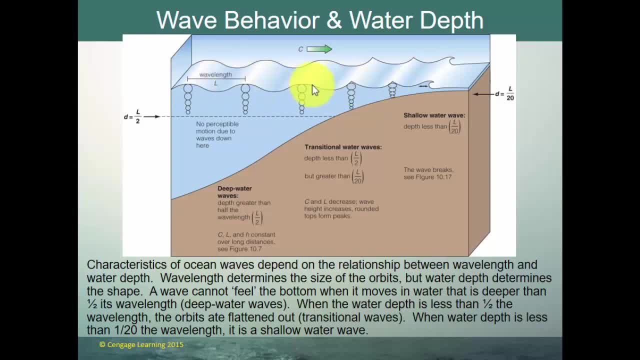 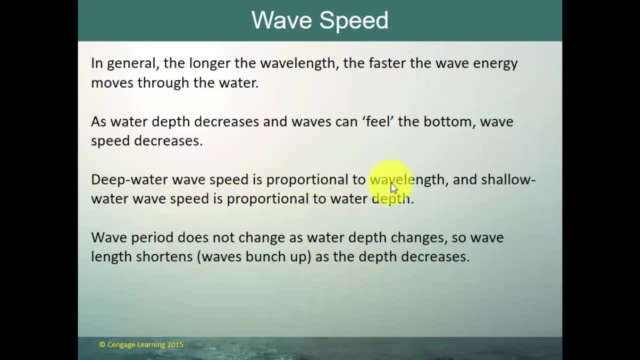 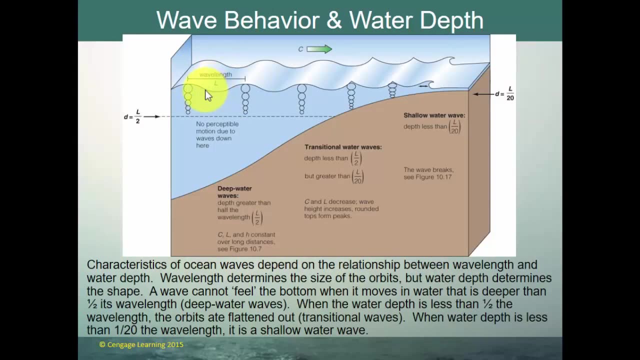 slows As these waves here feel the bottom. the wavelength between the wave also shortens as the wave approaches shore. So deep water wave speed is proportional to the wavelength, and shallow water wave speed is proportional to the depth. Again, the speed of these deep water waves has. 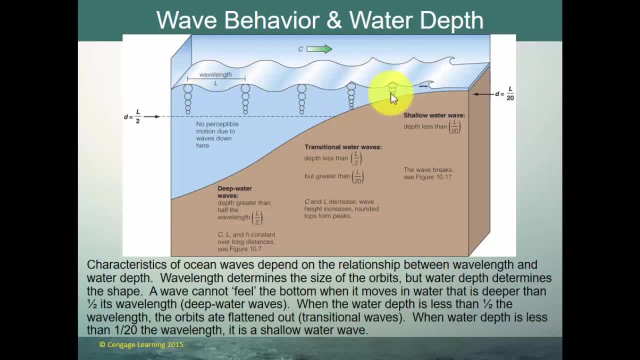 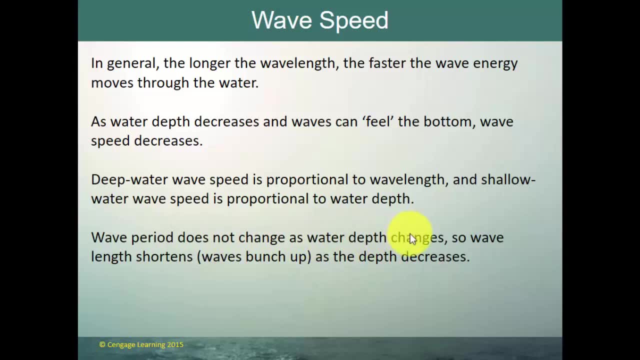 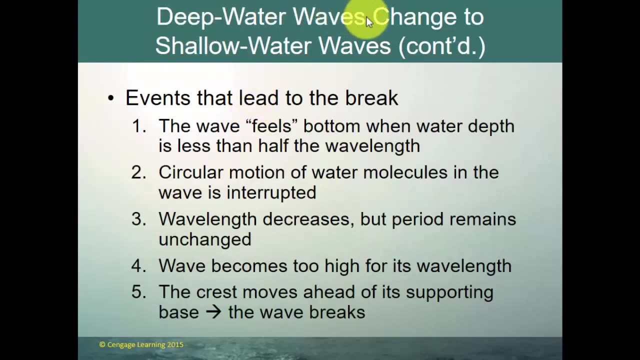 to do with the wavelength. The speed of these shallow water waves has to do with the water depth. Wave period does not change as water depth changes. so the speed of these deep water waves changes. So wavelengths shorten, waves bunch up as the depth increases, So deep water waves change. 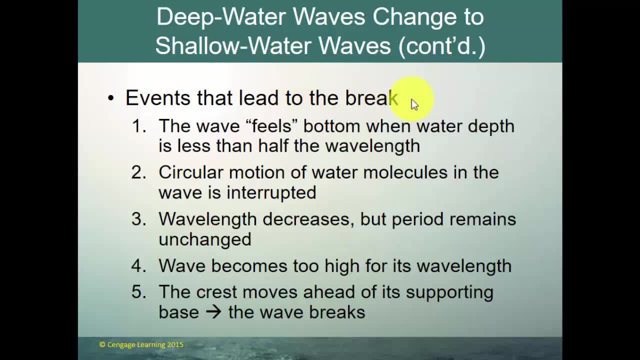 into shallow water waves. These are the events that lead the wave to break. First, the wave feels the bottom when the water depth is less than 1 half the wavelength. Second, the circular motion of the water molecules in the wave is then interrupted. Wavelength decreases, but the period 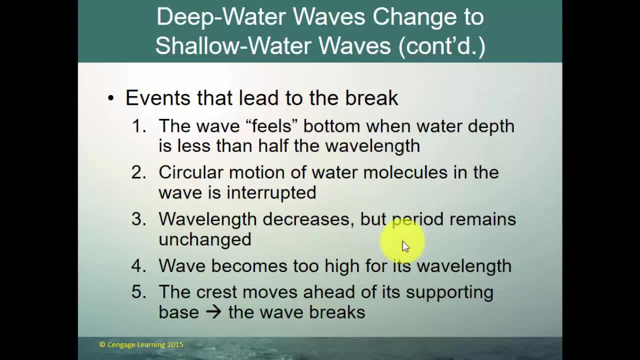 remains the same- That was the last point of the previous slide. The period, the number of wave crests that pass a point remains the same, but the wavelength decreases. Waves become too high for the wavelength, meaning the top of the wave becomes too high and the crest will move ahead. 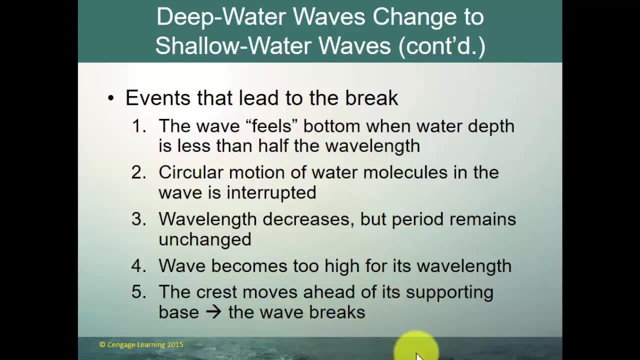 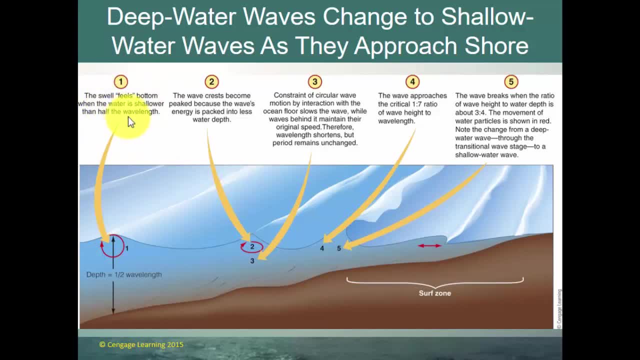 of its supporting base, causing the wave to break. So here that is graphically illustrated: The swell feels the bottom when the water is shallower than half the wavelength. So here it's half the wavelength, and the wave begins to feel the bottom when the water is shallower than half the wavelength. 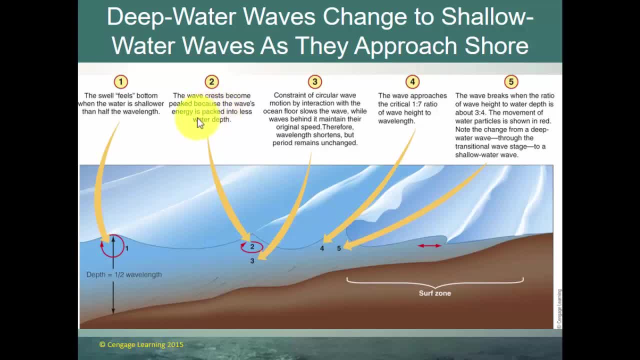 fuel the bottom. The wave crest becomes peaked because the wave's energy is packed into less water depth. So it pushes it up and it becomes peaked. These orbitals become more elliptical Constrain of circular wave motion by interaction with the ocean floor slows the wave, It slows down. 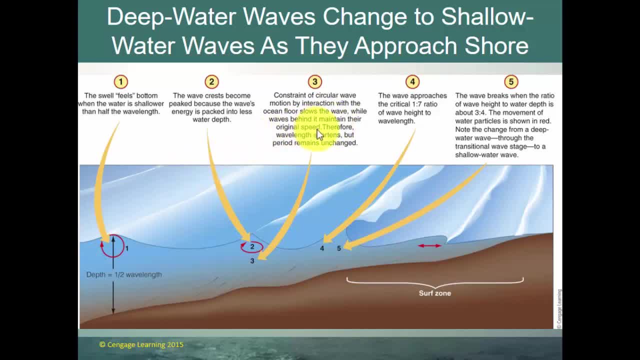 while the wave behind it maintains the original speed. Therefore, the wavelength has to shorten. The distance between the waves becomes shorter. That's like when you're standing in the surf zone: The waves are closer together than they are out in the open ocean. The period remains unchanged. 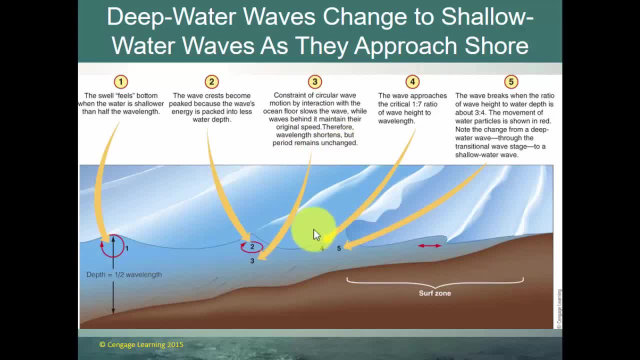 The number of waves that will pass a certain point at a time remains the same, but the distance between them shortens up. At four the wave approaches the critical one to seven ratio of wave height to wave length. When it passes that ratio, the top of the wave literally continues. 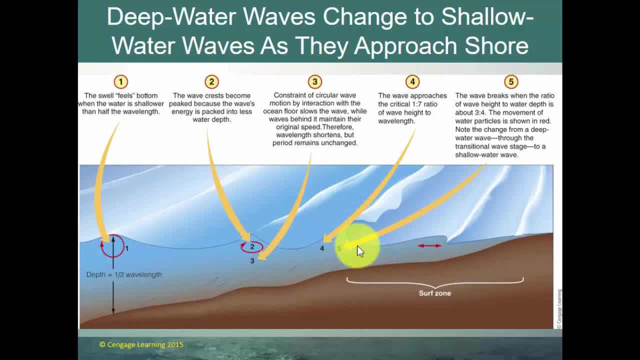 moving faster than the bottom of the wave. So at five the wave breaks and the ratio of wave height to water depth is about three to four. The movement of the water particles is shown in red here. Note the change from a deep water wave. 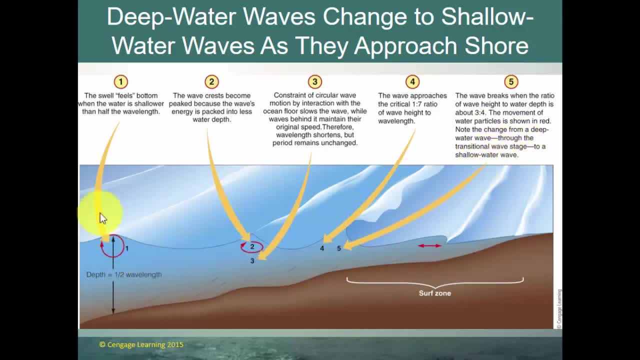 through the transitional wave stage to a shallow water. So here it's a circle, here it's an elliptical and here the water is literally moving back and forth after that water breaks, and this is after that wave breaks, and this is known as the surf zone. So two different types. 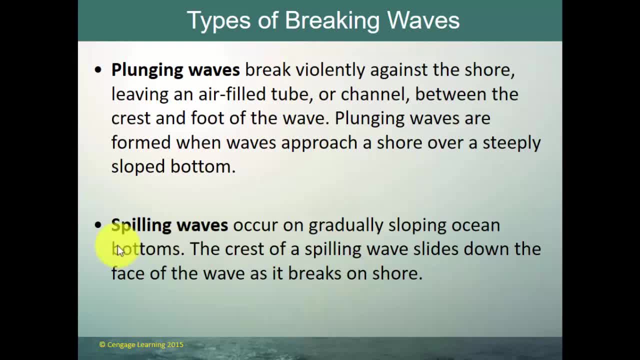 of waves. Waves that we typically see here in Florida are spilling waves. They just sort of crumble over one another. And then we have plunging waves, the waves that sort of pitch out and create well, the tube, as surfers call it, or sort of pitch out and are more hollow, So plunging. 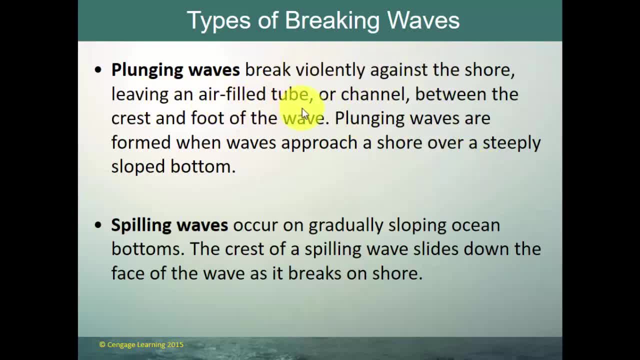 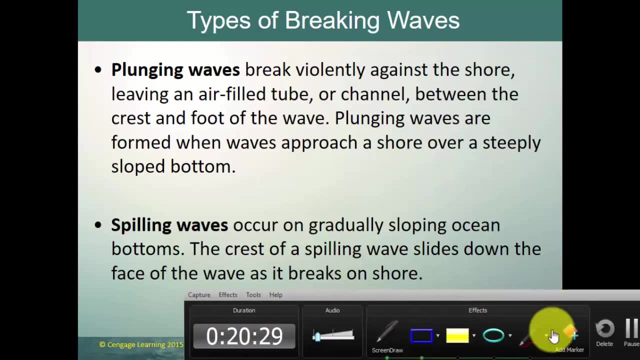 waves will break violently against the shore, leaving an air-filled tube, the tube that surfers talk about, or a channel between the crest and the foot of the wave. Plunging waves are formed when waves approach a shore over a steeply sloped bottom, So essentially, the plunging wave. 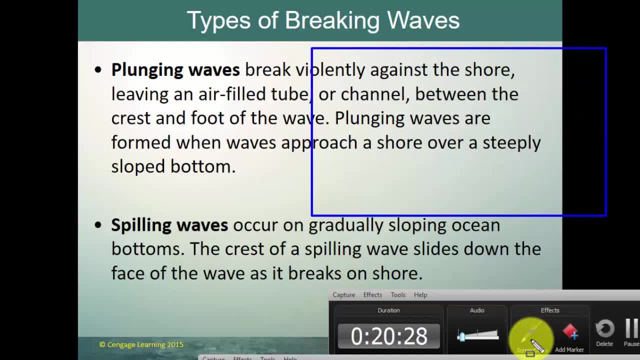 is this it So? if this is, If this is the bottom, as the wave comes in like this, if it's steeply sloped, the top of the wave gets thrown out, while the bottom of the wave literally stops and you get that. 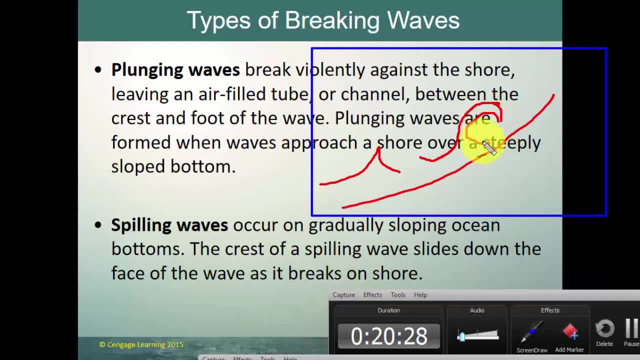 plunging wave- Not the greatest picture in the world, but you get that plunging wave. That's the two. If you have a shallow slope- it's a more gradual slope, it's a more gradual slope like this- then those waves will tend to crest and they'll just sort of crumble down and 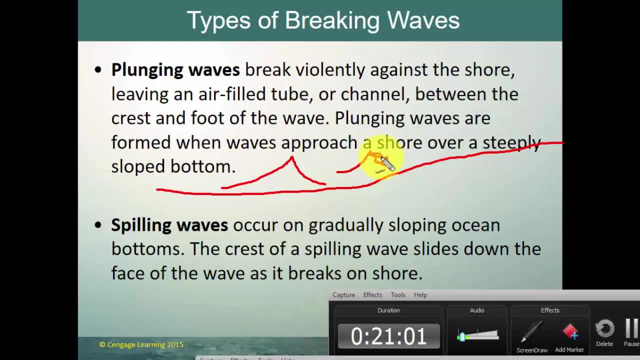 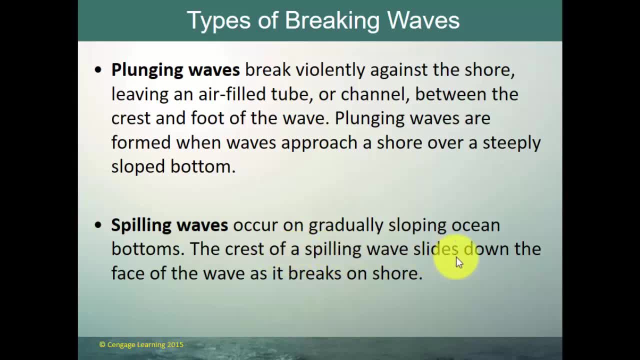 that's kind of what we see here in Florida, where the wave it doesn't plunge, it just sort of spills over and crumbles down. So spilling waves occur on gradually sloping ocean bottoms. The crest of a spilling wave slides down the face of the wave as it breaks onshore. 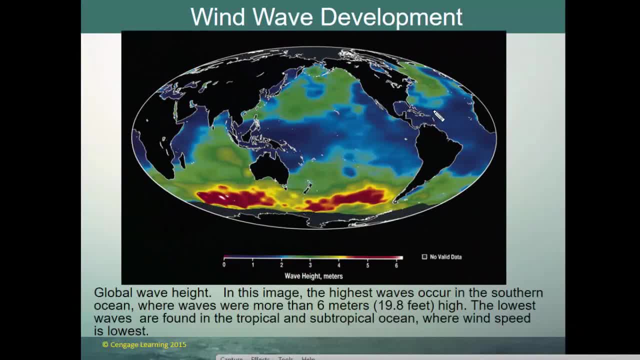 All right. So where would you typically find the biggest waves? You'd find them where you have the highest winds, and you have the highest winds where you have the mid-latitude westerlies moving across the Pacific and the Atlantic Ocean and then, very specifically, the westerlies moving across the Southern Pacific, the Southern 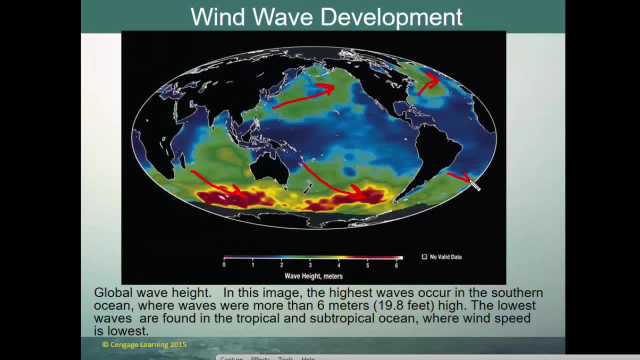 Indian Ocean and even, to a lesser degree, the Southern Atlantic Ocean. because these southern oceans the winds are not impeded by land. There's a lot of open ocean. the winds are only slightly impeded by land here, not impeded by land. 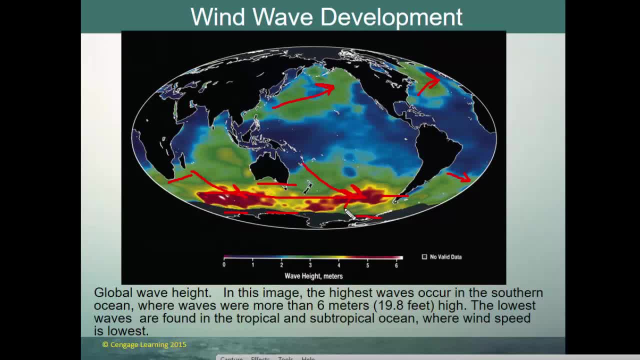 So your highest winds are across this section of the Southern Ocean and it's that section of the Southern Ocean where you do see those wave heights up to five to six meters. So in this image the highest waves occur in the Southern Ocean, where the waves are. 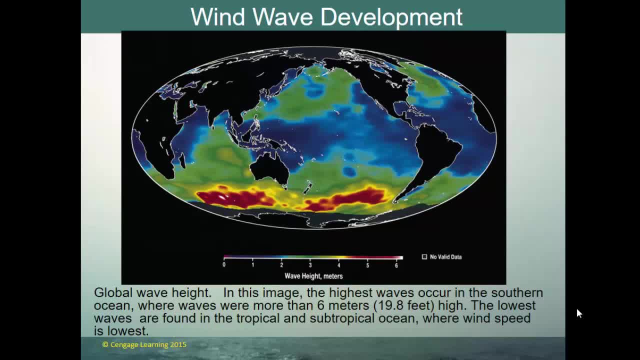 more than six meters, 20 feet or so high. The lowest waves are found in the tropics. Remember, the tropics are where we have the doldrums. These are the where not much happens. There's not a whole lot of wind and therefore there's not a whole lot of waves. 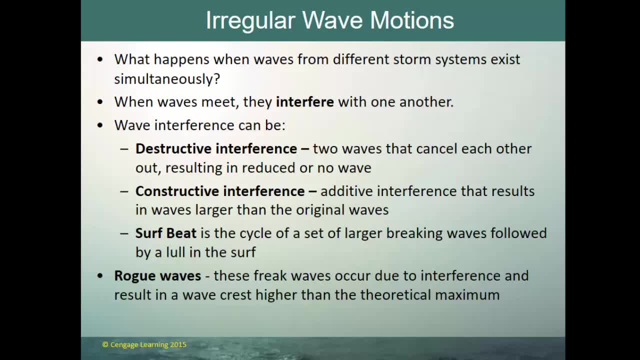 What happens? What happens? Well, all the storm systems exist simultaneously. If you think about the open ocean, you might have wind coming from the Northern Atlantic Ocean, maybe some wind coming from a tropical system down closer to the Caribbean, and all these different winds will likely generate different types of wind waves. 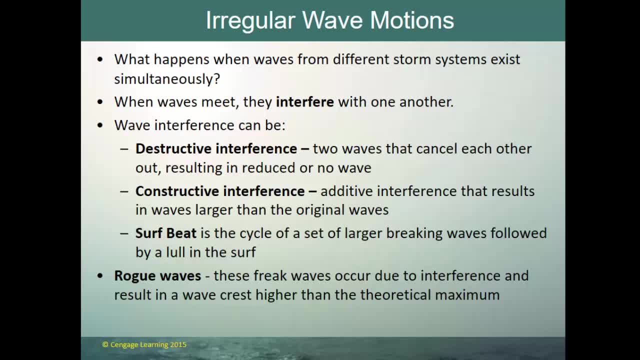 So what happens when different waves and different storm systems interact? Well, when they meet, they interfere with one another, and there's two types of interference: destructive and constructive. Destructive interference is when two waves that actually cancel each other out, resulting in a reduced or no wave at all. so two waves can 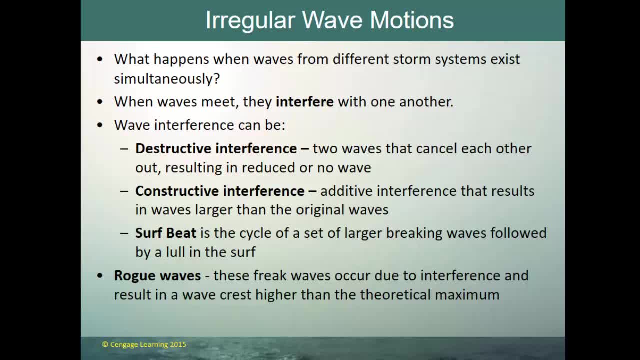 come at each other from two different directions and really serve to cancel themselves out. more often we see constructive interference, where there's additive interferences, where the waves actually add to each other and that results in waves that are larger than the original waves. but it's going to be a combination of both, depending on how and what angles the winds and the waves. 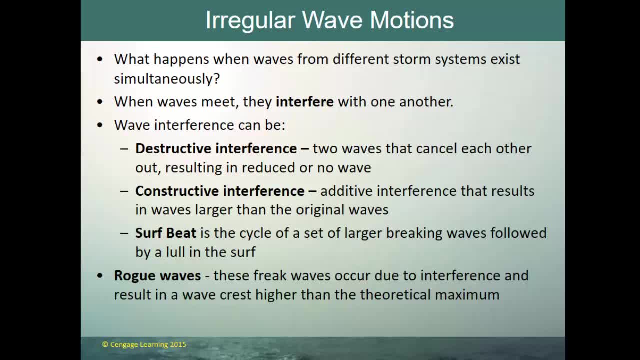 meet at, and so what you get is this: this offset of lots of different size waves moving to the same region, and that cycle of larger and smaller waves that we hear in the breaking surf is what's known as the surf beat. so surf beats not just a type of music, but it's actually a scientific term referring 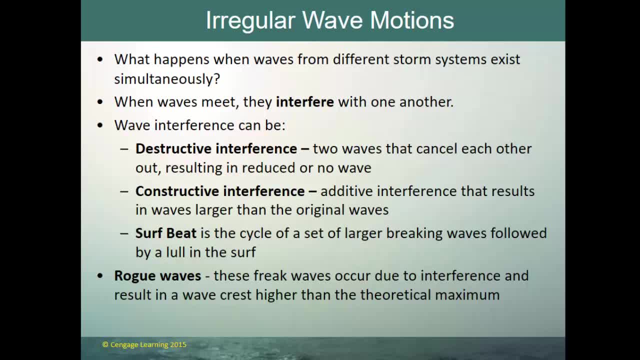 to the cycle of a set of larger breaking waves followed by a lull in the surf and then smaller breaking waves. now, if you have lots of constructive interference, you can get these freak waves that that occur, that become gigantic and those are rogue waves. and that is when you get a wave, the crest is higher. 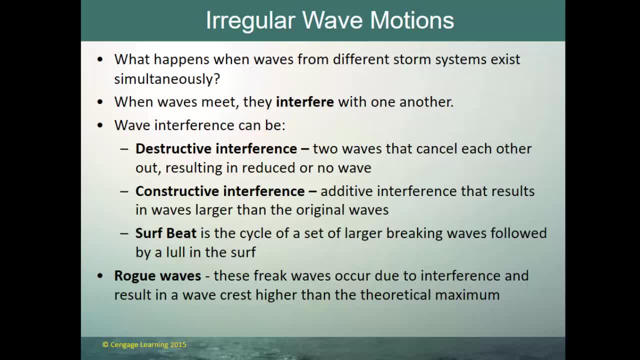 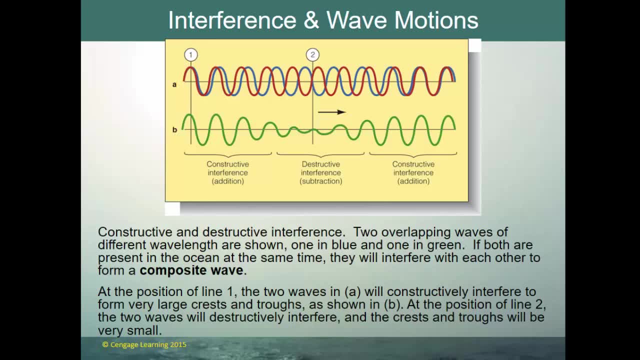 than the theoretical maximum of those waves, and you mainly see that again down in the southern ocean. so constructive interference and destructive interference. two overlapping waves of different wavelengths are shown, one in blue and one in green. if both are presented in the ocean at the same time, they'll interfere with each other to form a composite wave. so the composite wave is 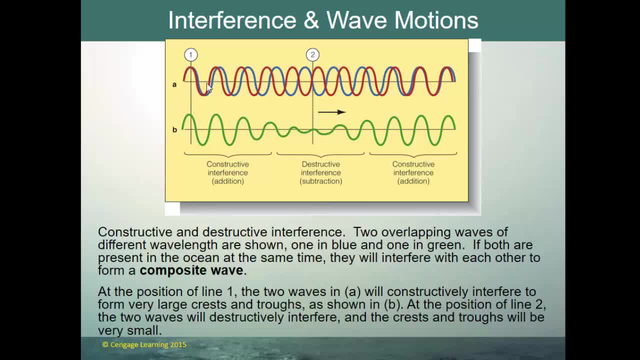 actually the one that's going to be in green here, the two different waves and red. so the different waves have essentially different wavelengths. so there are periods of time when they're synced together and they have constructive waves, and periods of time when they're they're synced apart and you create destructive interference and so you get additive. 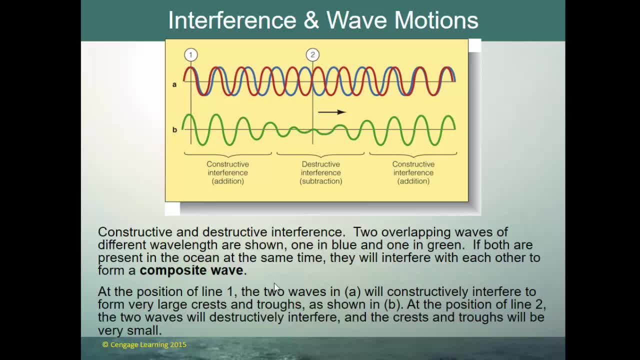 situations here and then destructive situations here. at the position of line one, the two waves will constructively interfere with each other to form large crests and troughs. and then at b, at the position of line two, the two waves will destructively interfere and the crest and drops will be much smaller. so that's the result of both constructive and 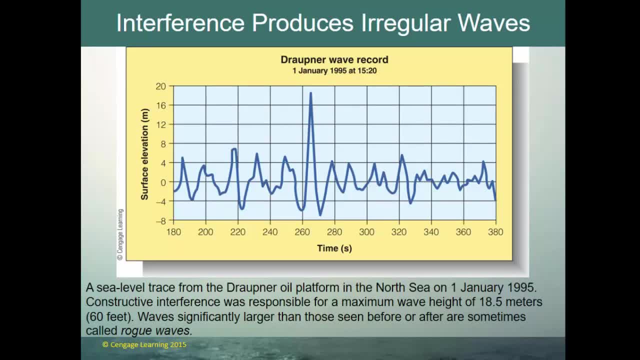 destructive interference. so here's the sea level trace uh, at this oil platform in the north sea back in 1995 where constructive interference is responsible for a wave of almost 19 meters. so we're talking 55 to 60 feet uh, and you can see you had pretty typical surf beat with some constructive 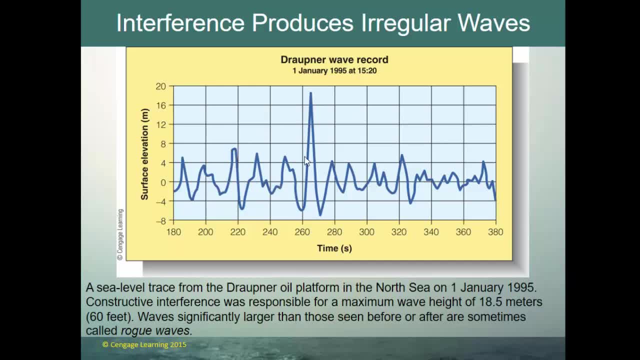 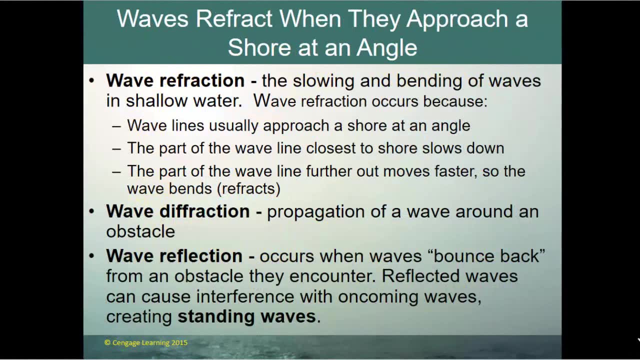 interference, and then destructive interference somewhere in between, and then some constructive, tremendous peak of this wave, and that's one of those rogue waves. Three things that happen to waves, particularly as they approach the shore: refraction, diffraction and reflection. Wave refraction: the slowing and bending of 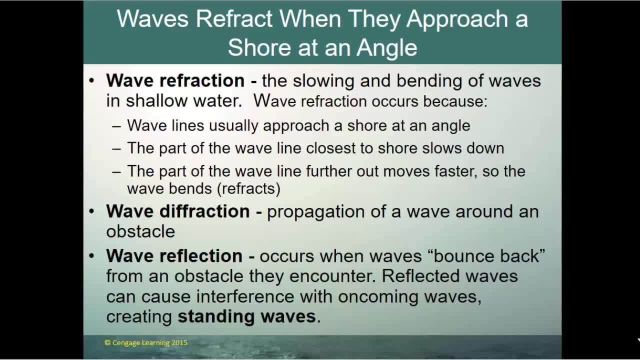 waves in shallow water. Wave refraction occurs because waves usually approach shore at an angle. The part of the wave line closest to the shore slows down as it can feel the bottom. The part of the wave further out moves faster, so it catches up to and passes the part of the wave line in the shallower water and 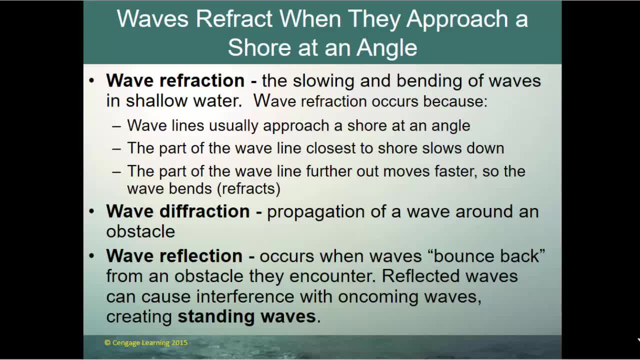 that causes the wave to bend or to refract. Diffraction is when a wave literally propagates around an obstacle. essentially for the same reason, A straight wave hits an obstacle at the center of the wave. where it hits the obstacle, the water is shallower and it causes the wave to literally bend around. 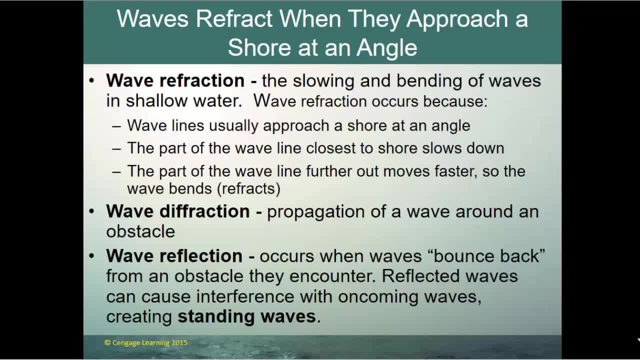 that obstacle and that is diffraction. And you also see reflection. when a wave bounces back from an obstacle that it encounters, Reflective waves can cause interference with oncoming waves and create standing waves. Think about the last time you were at the ocean when the wave rolled up the 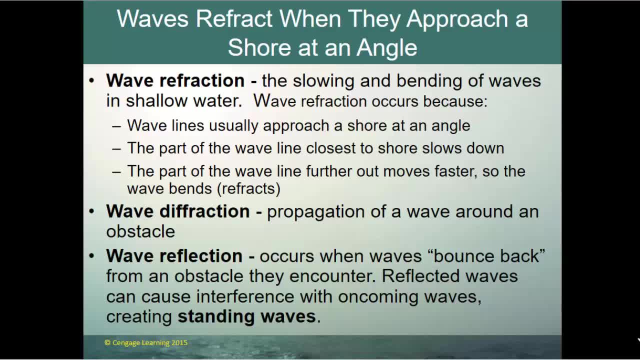 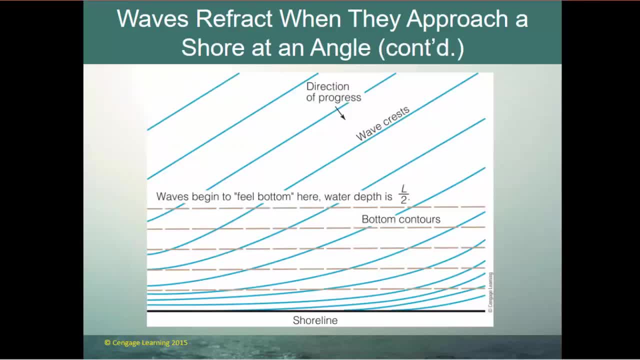 seashore, then rolled back down. Sometimes it creates a little standing wave in just an inch or two of water. That is interference, creating that standing wave. So this is what that looks like. The wave progression is coming in at this angle. So this is the shoreline down here and this is the angle You get a nice. 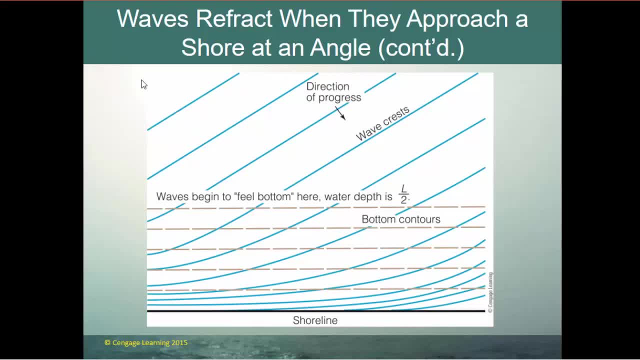 let's say this is a shore facing east and north wind blowing. a northeast wind swell in This wave propagates along at the same speed Again. once the wave begins to feel the bottom where it is, the depth is half the wavelength. then the wavelength begins to shorten and the wave starts to slow down. But these waves 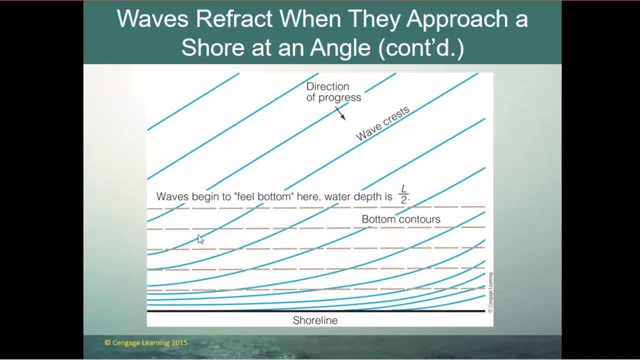 are moving at the same speed and it literally causes these waves to bend and also causes them to essentially come in almost straight parallel to the coastline. So That's what we typically see at the beach: is waves coming straight in because, as they've felt the bottom, they will begin to bend and straighten out. 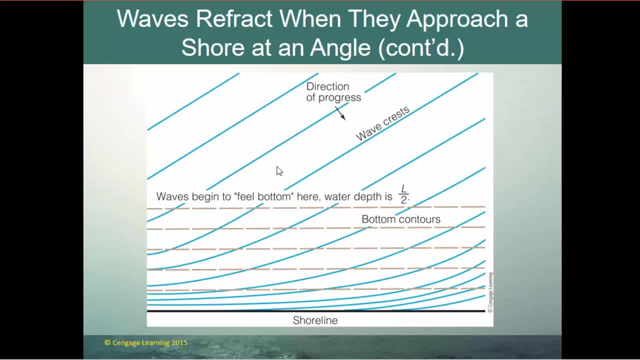 And so where you get waves coming in at a sharp angle to the beach is where the water depth is deep and then becomes shallow very abruptly. Here in the Atlantic Ocean, on the east coast of Florida, the ocean bottom gradually slopes out, and so you have enough time for these waves to literally refract. 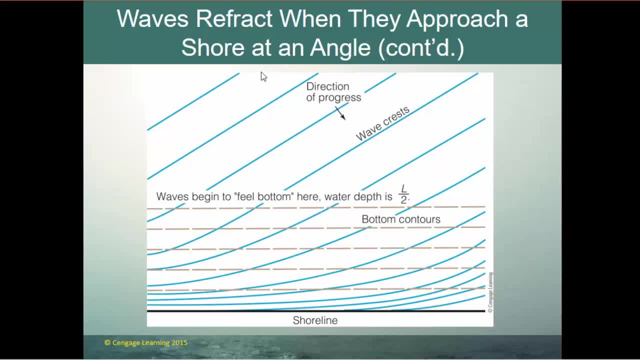 and then come in straight to shore. But this is refraction. Here the water's deeper, here it's shallower. Where it's shallower, the wave moves slowly and the wavelength decreases. Here the wavelength is the same and the wave is moving more quickly. 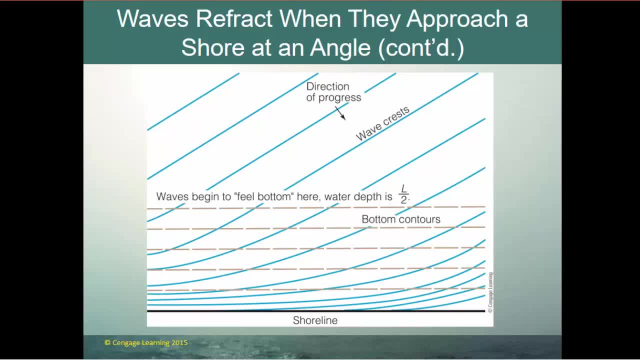 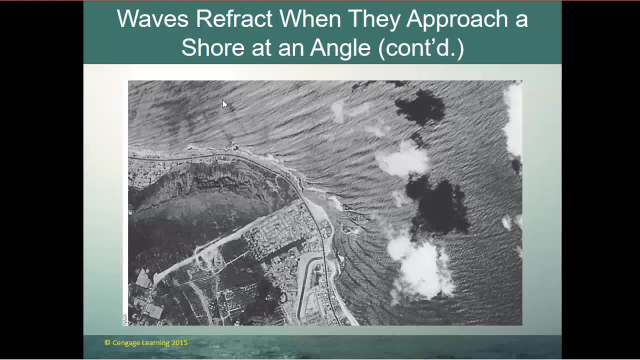 and it causes the wave to bend, to refract as it approaches shore And you can see that refraction as it comes along the shoreline. Here the waves are coming in, This is the angle they're moving and as they come along the shoreline they refract and bend into the shoreline. 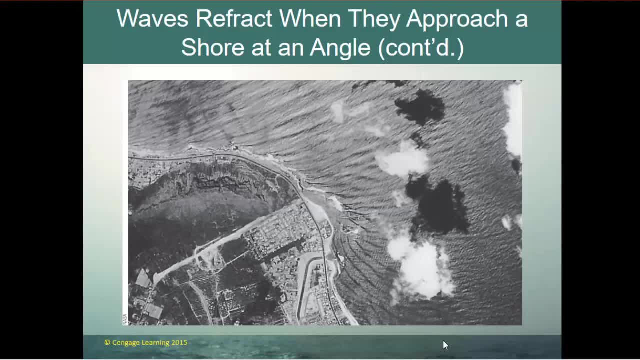 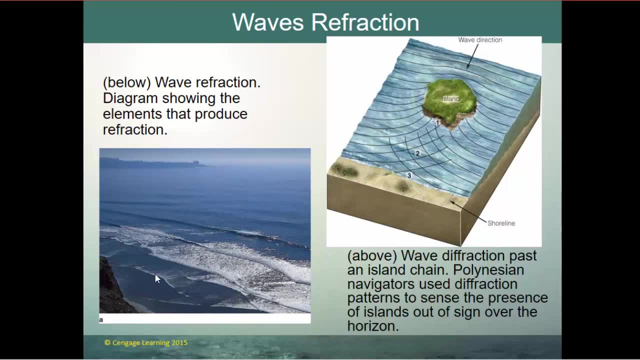 where in most cases they're almost coming in parallel to the shore in every location. So wave refraction again: Waves coming in at this angle here and they refract and bend in so they're coming almost straight into the ocean. And here's the diffraction. 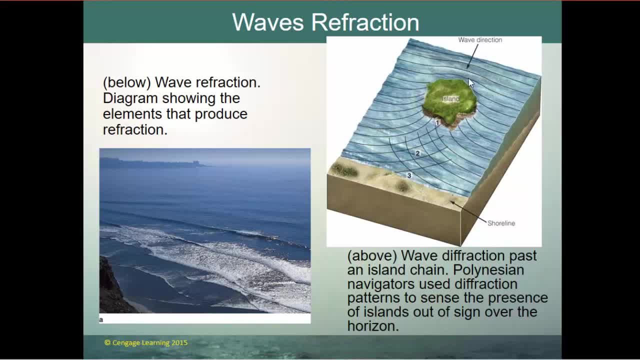 When the waves are coming in straight here. as they hit this little island and get shallower, the waves begin to slow down and so they bend around just like there were if it was just a straight coastline. and then over here you get this constructive and destructive interference. 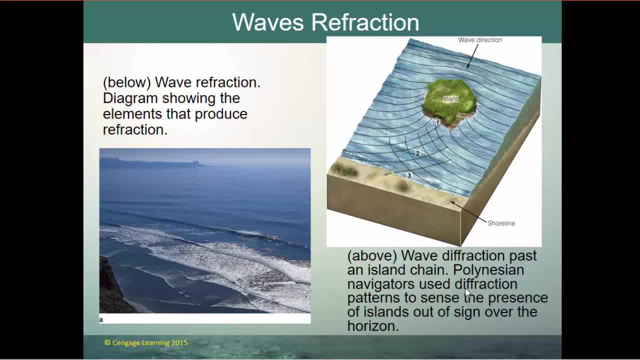 So wave diffraction past an island chain. Polynesian navigators use diffraction. They use these patterns to sense the presence of islands out of sight from the horizon. So if you were a canoe coming along this way and you didn't see this island, 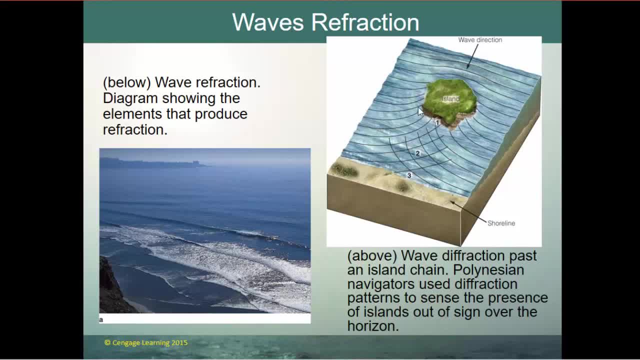 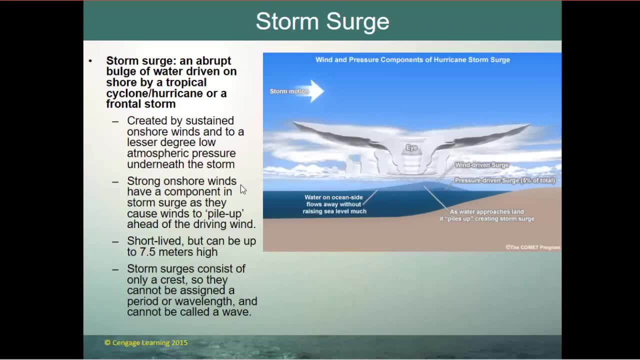 you would get this constructive interference and you know that somewhere off in the distance there was an island. So that is going to be your diffraction and your refraction, And then again you also have the reflection. So storm surge is an abrupt bulge of water. 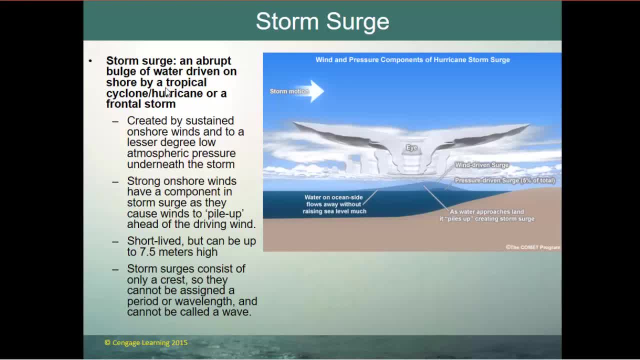 So it's kind of like a wave, but it's a bulge of water driven onshore by a tropical cyclone, hurricane or frontal storm, So it's created by sustained onshore winds, The storm motion and the wind motion is in this direction. 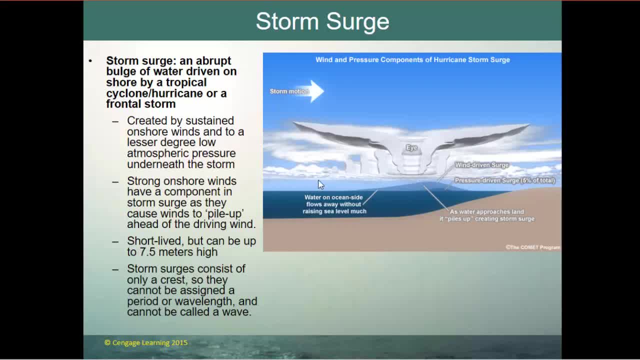 coming from offshore to onshore and it literally pushes up a mound of water. Now, there was a time when we thought that the low pressure of the hurricane may have lifted up that mound, but we now know that pressure-driven storm surge is only about 5% of the total. 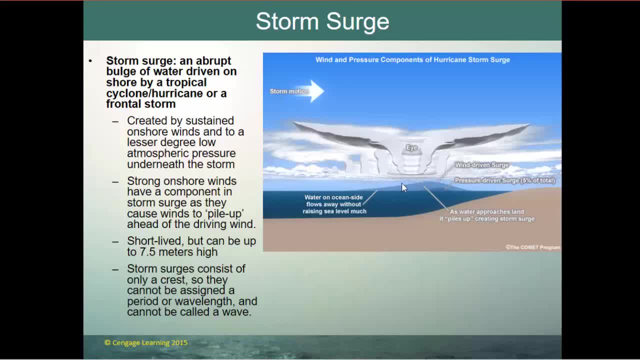 All the rest of it is wind blowing that water and causing it to pile up- Strong onshore winds. Strong onshore winds have a component in storm surge, as they cause winds to pile up ahead of the driving wind. They can be very short-lived but they can be up to. 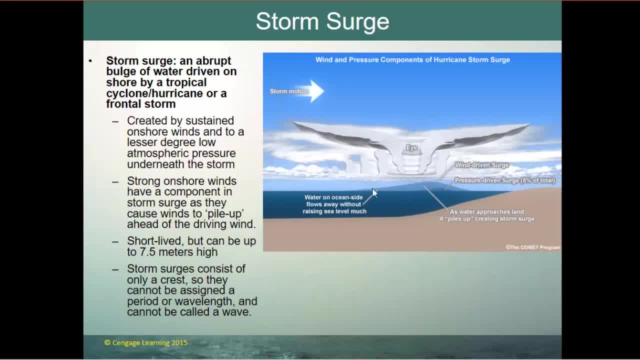 so 7.5 meters, we're talking 20 to 25 feet. It can raise the level of the ocean. So this mound is almost like a tide coming in and raising the level of the ocean because the breaking waves caused by this wind. 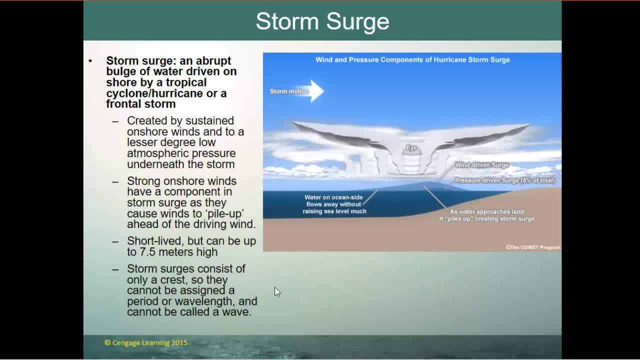 literally break on top of the storm surge. So storm surge consists of only a crust, so they really can't be assigned a wavelength or a period- not really called a wave either- but it definitely brings the water up and causes serious damage. As a matter of fact, most of the damage from hurricanes 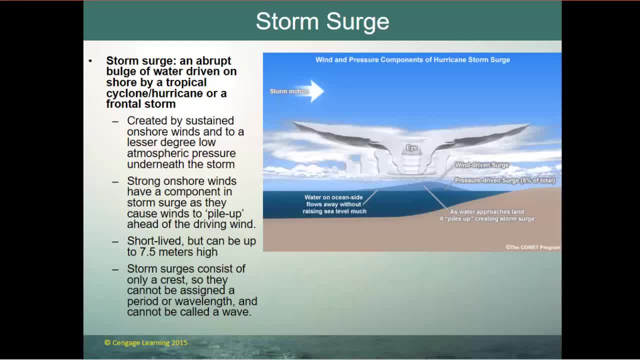 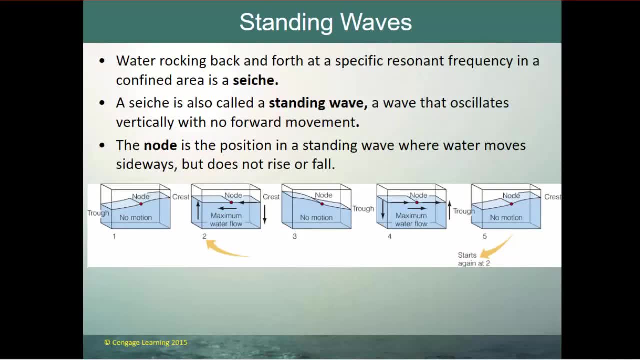 and deaths from hurricanes is caused by the storm surge. Standing waves, Water rocking back and forth at a specific frequency in a confined area is called a seiche, and it's also known as a standing wave. Now you can get standing waves in rivers. 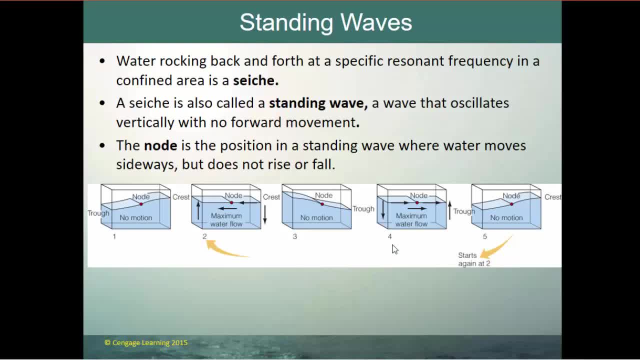 where the water is moving along and for some reason it gets diffracted Off of an obstacle- not diffracted, but reflected off of an obstacle- and moves back down. You can also get a standing wave in the situation where you have the ocean wave moving up the seashore. 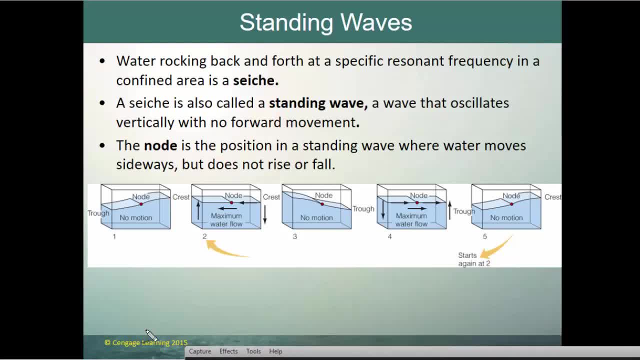 So I'll try and draw a couple of these for you. If this is your seashore and your wave is moving up it and it gets to a point where it stops and moves back down, this motion back down can create a standing wave right here. 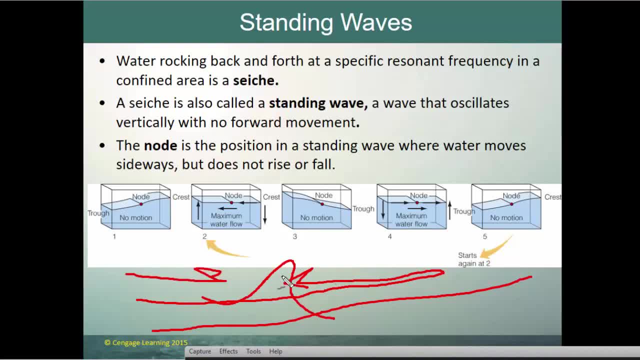 where there's water motion in and there's water motion out and you get the standing wave. You can also get that in a river situation where the river is flowing along like this, but some obstacle- maybe there's a boulder here. 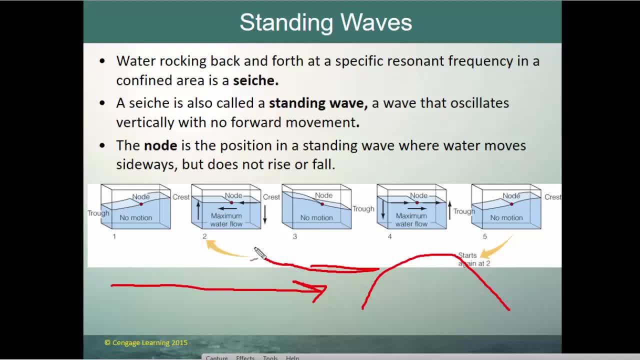 causes water to bounce back off and again you'll get that standing wave in one spot. So that's what standing waves are, but we also have these standing waves that happen in enclosed basins, So maybe this is a lake or a tidal basin. 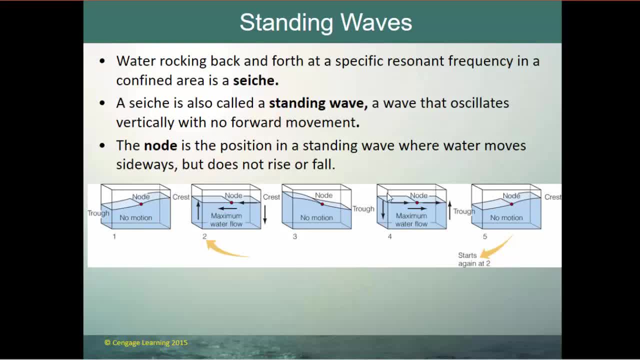 but it's going to be an enclosed basin and water is going to be in an enclosed basin and it's going to oscillate back and forth in this closed basin and essentially it's a standing wave where the water goes up and down. 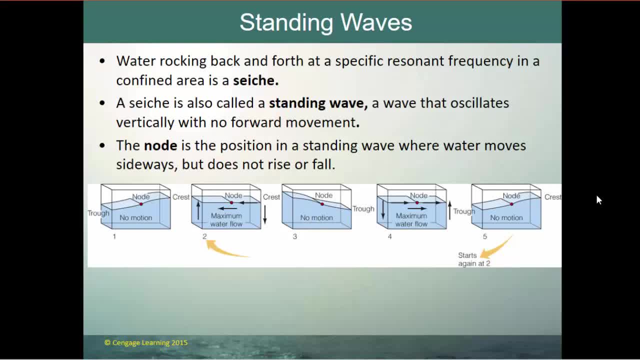 and up and down, So water rocking back and forth at a specific frequency in a confined area is called a seashore. A seashore is also known as a standing wave, a wave that oscillates vertically with no forward movement, Just like the waves I just drew for you. 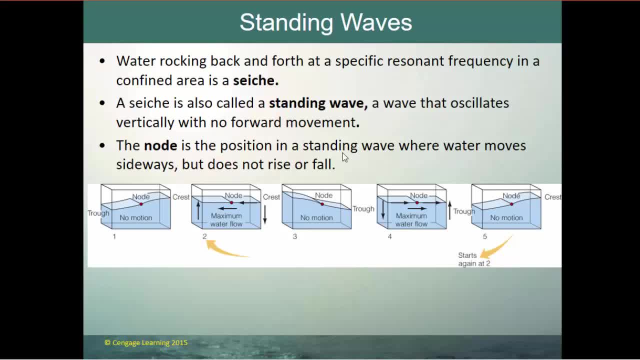 they go up and down but they have no forward movement. The node is the position of a standing wave, where water actually moves sideways but does not rise or fall. So this is a standing wave going through its whole sequence from one to five. 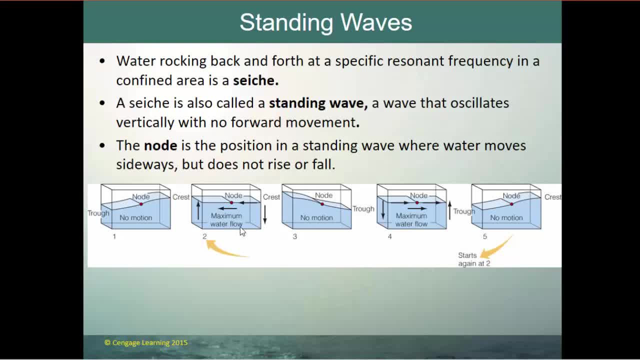 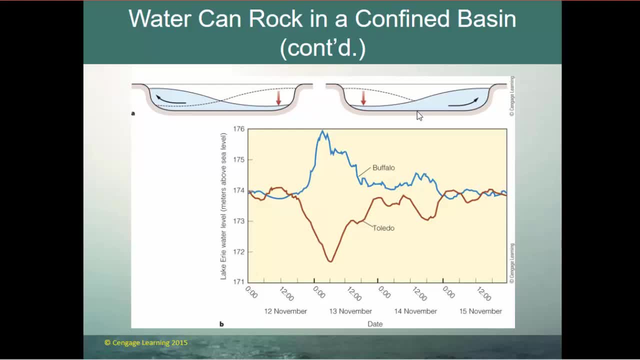 and then back to two again. So it just is up and down. up and down motion but no back and forth motion. So water can rock back and forth in a confined basin, and this happens sometimes in the Great Lakes where at one side of the Great Lake you have high water. 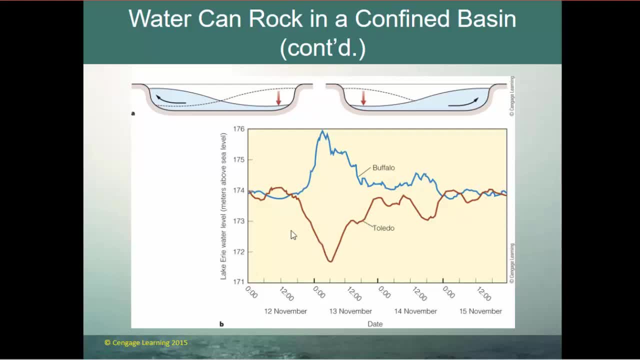 and at the other side of the Great Lake you have very low water, And so that's an example of that standing wave. The Great Lake represents the standing basin, but wind blowing over that Great Lake for a long period of time can create a wave where water pushes to one side. 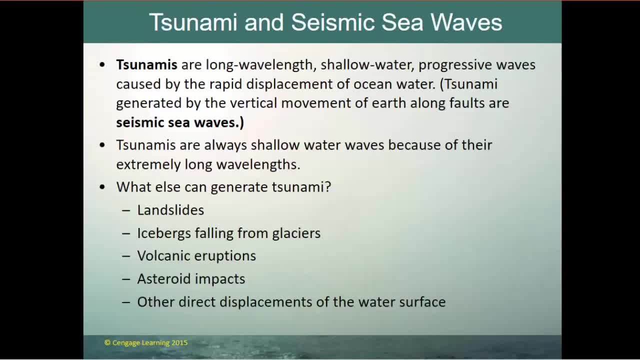 and then essentially sloshes back to the other side. Tsunamis and seismic sea waves. Tsunamis are very, very long wavelength shallow water. shallow because their wavelength is so long they're essentially always in shallow water. 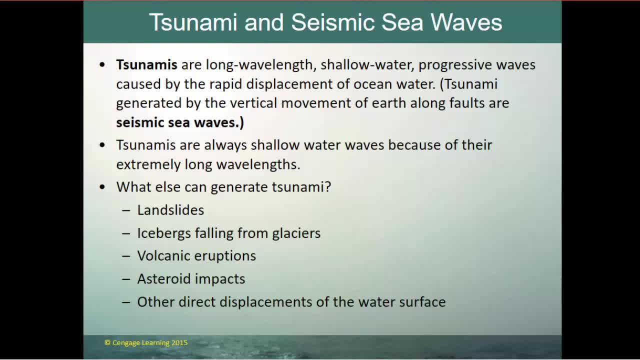 even in the deep ocean. They're progressive waves caused by the rapid displacement of ocean water. Tsunamis are essentially created by the vertical movement of Earth along faults and they're called seismic waves. So this is your ocean basin. That's the surface. 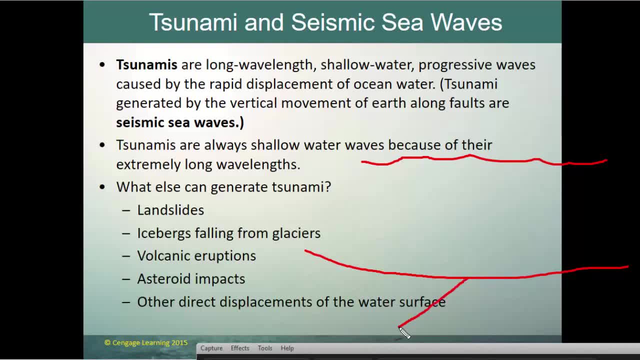 This is the sea bottom and there's a fault along that sea bottom, right here, And the pressure of that fault is pushing this part of the rock up and this part of the rock down. Maybe it's a convergent fault, boundary So over many, many, many, many thousands of years. 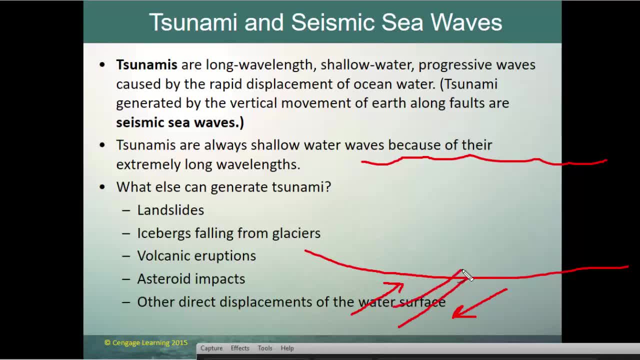 this pressure builds up, pressure builds up and then suddenly, one day, this fault gets forced up and this sea bottom actually gets pushed up. So it looks something like this: Well, it displaces all of this water and all that water gets pushed up. 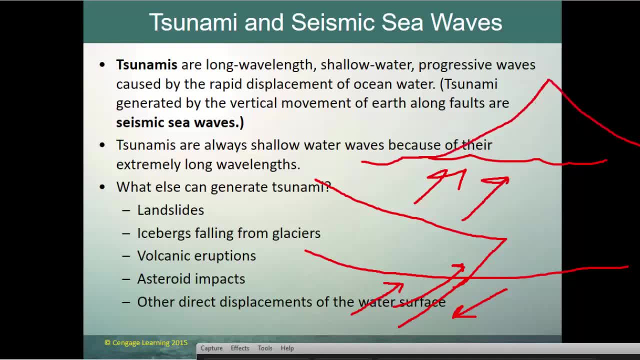 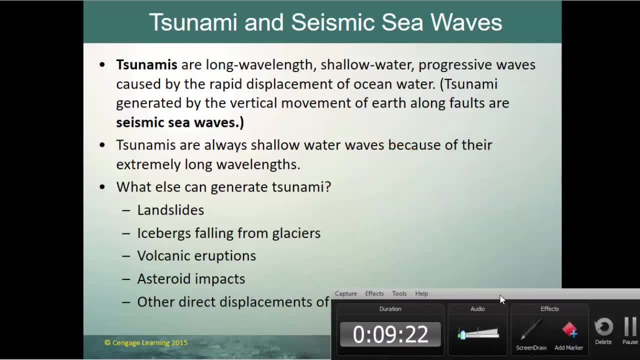 and that displacement of water causes your tsunami, your initial tsunami, to form and then propagate away. Now they'll also back up a smaller wave, but the major tsunami is going to move in that direction. So a seismic sea wave or a tsunami. 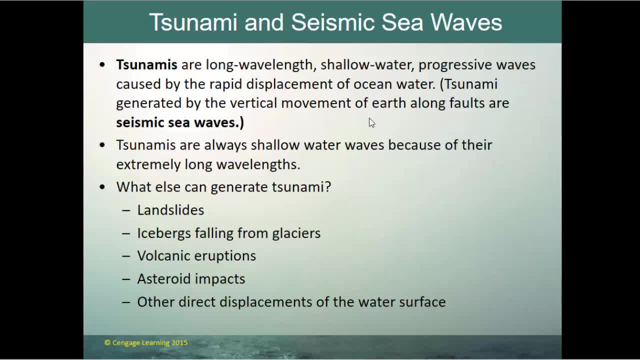 is generated by the vertical movement of Earth along faults and they are seismic sea waves. Tsunamis are always shallow water waves because they're extremely long wavelengths And you can also get a tsunami generated by a landslide. So a lot of Earth. 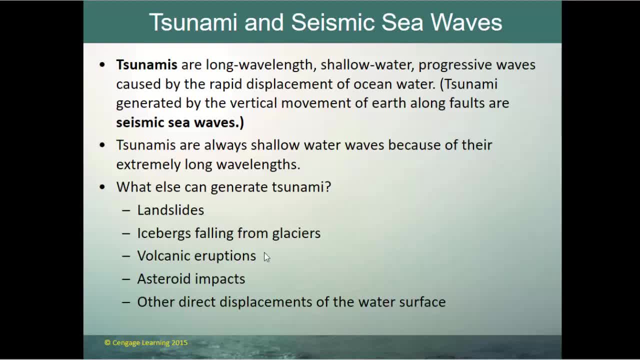 coming down the side of a mountain into the ocean. icebergs calving: when icebergs are part of the ice sheet and they fall off into the water, it's called calving. So icebergs falling from glaciers, volcanic eruptions, asteroid impacts. 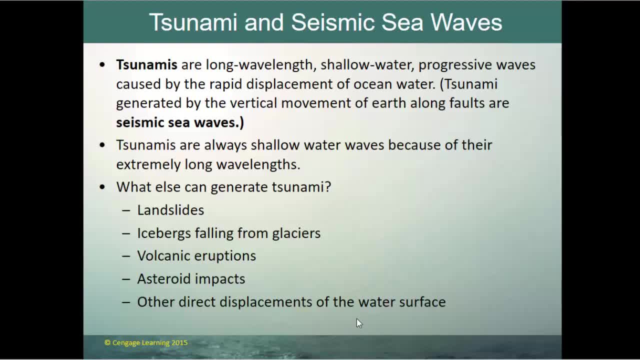 any direct displacement of water will cause a tsunami And they are devastating, much like storm surge They create. you know most of the deaths that you would attribute to ocean waves. Most recently we had the Indian Ocean tsunami from an earthquake back in December. 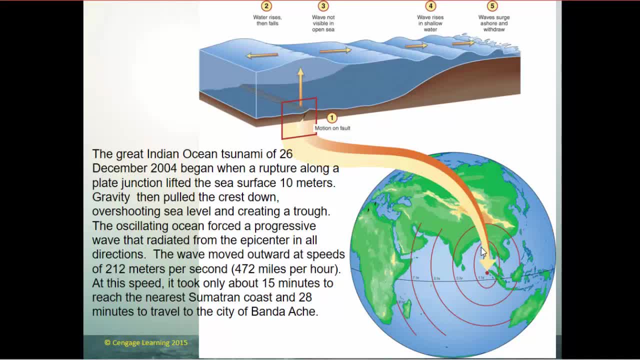 2004,. and it was exactly the situation I showed you. We had a convergent plate boundary where this plate was moving up into this plate and once it was forced under it- and here's the fault- it pushed this land up and it created that ocean wave. 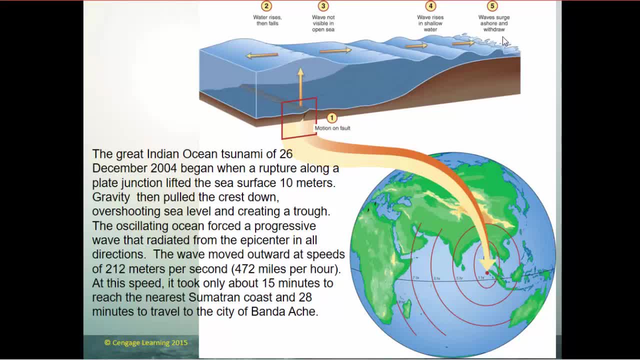 Now the main wave moved away, but also the tsunami moved toward land, So it happened just offshore Jakarta and so this wave washed up in Jakarta, creating a tsunami there. So the Great Indian Ocean tsunami, 26 December 2004,, began when a rupture. 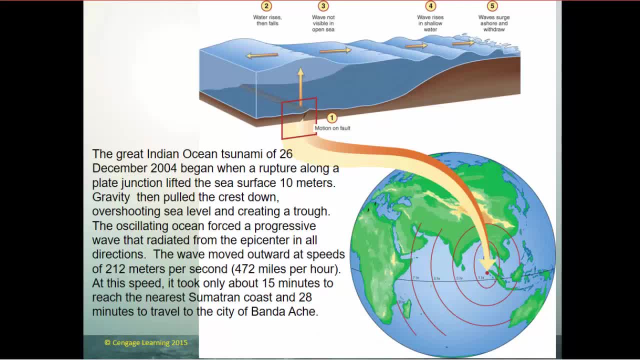 along a plate junction lifted the sea surface about 10 meters Gravity. so the first thing that happens, the sea, it gets lifted up. So that's the disturbing force. What's the restoring force? Gravity is the restoring force, So it pulls it back down. 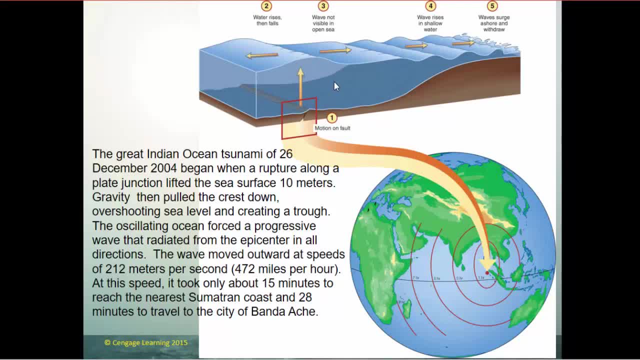 but it doesn't necessarily pull it just back down to sea level. Gravity pulled it further down than sea level and so that it needed to be restored back up, and it went up beyond sea level and then back down and back up. 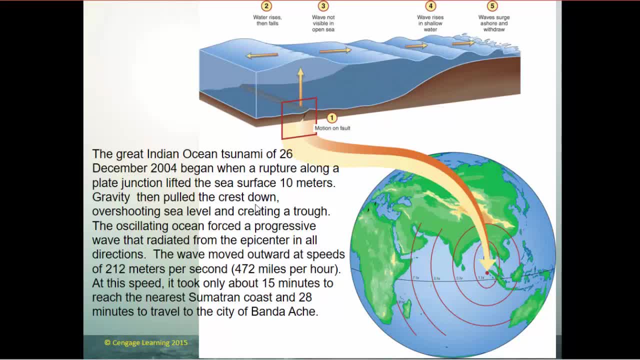 and then back down, And so that's how this displacement of water creates a wave. Gravity pulled the crest down, overshooting sea level and creating a trough. The oscillating ocean forced a progressive wave that radiated from the epicenter in all directions. 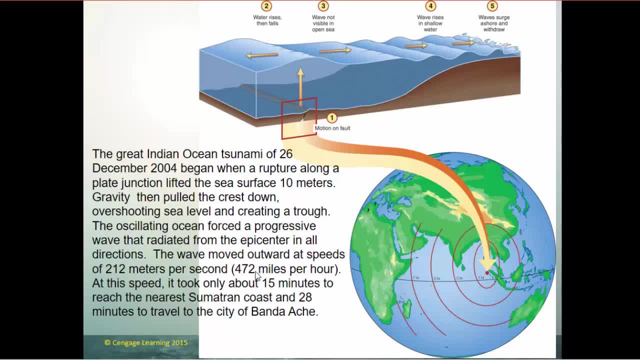 The wave moved outward at. this is astonishing: 472 miles per hour- That's how quickly it moved across the ocean because of the tremendously long wavelength. At this speed it took about 15 minutes to reach Sumatra and about 28 minutes to get across the Indian Ocean. 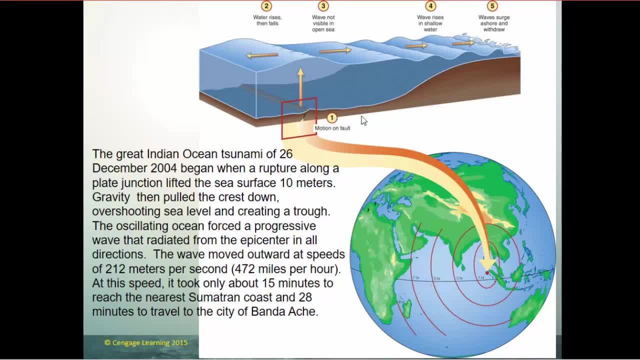 So this is a very, very classic scenario of a tsunami. Same thing happened in Haiti, with an offshore earthquake causing the displacement of the ocean and a tsunami radiated away from that area. All right, because tsunamis have extremely long wavelengths. 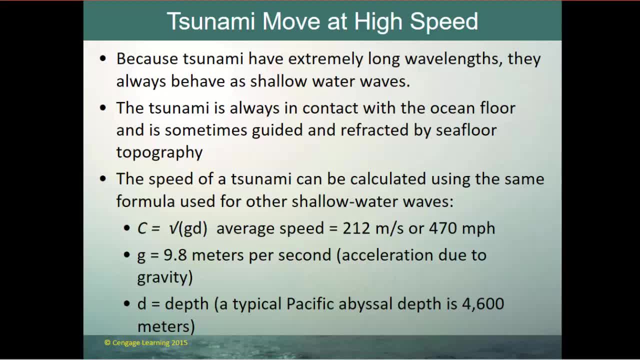 they're always in shallow waters, They always behave as shallow water waves. The tsunami is always in contact with the ocean floor, and sometimes it's actually guided and refracted by the seafloor topography. So the speed of the tsunami can be calculated using the same formula. 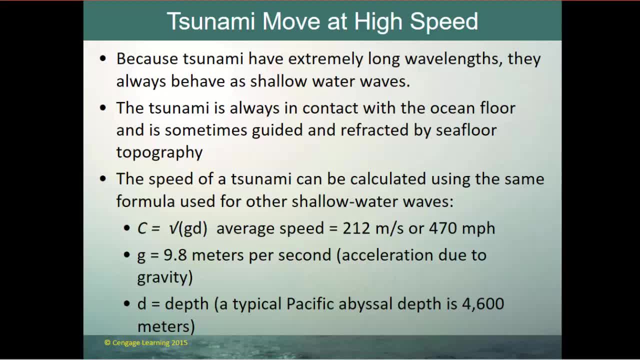 as for other shallow water waves, which that speed is the square root of gravity times the depth. So C equals the square root of gravity times the depth, the average speed of about 470 miles per hour. So your gravity is 9.8 meters per second squared. 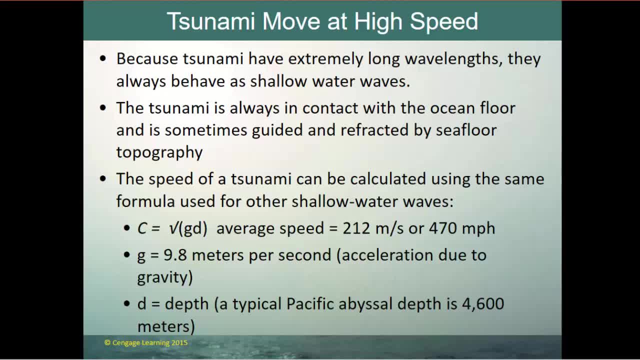 and the depth of the Pacific abyssal area is about 4,600 meters. So you multiply those two things together and take the square root and you get that average, the average speed of a tsunami of 212 meters per second, or 470 miles per hour. 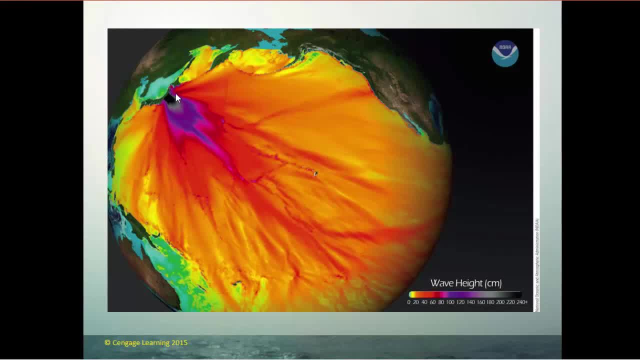 So here is the wave height again from the tsunami that happened, the earthquake that happened just off Japan, with the disaster with the nuclear power plant and the tsunami that radiated away from it because of that earthquake. So that's Japan, the Lucian Islands. 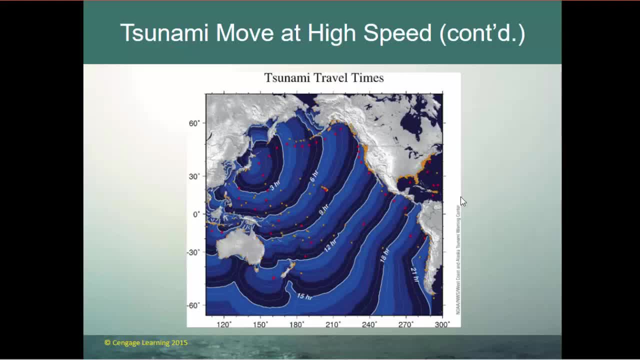 and the west coast of the United States, And that's what it looked like in terms of travel times. how long it took that ocean wave, that shallow water wave, that tsunami wave, to reach even as far south and east as the south coast of South America. 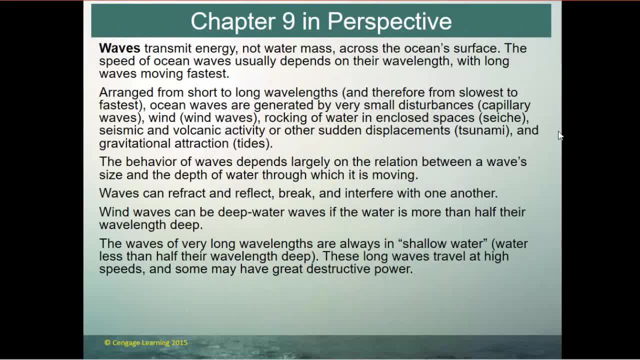 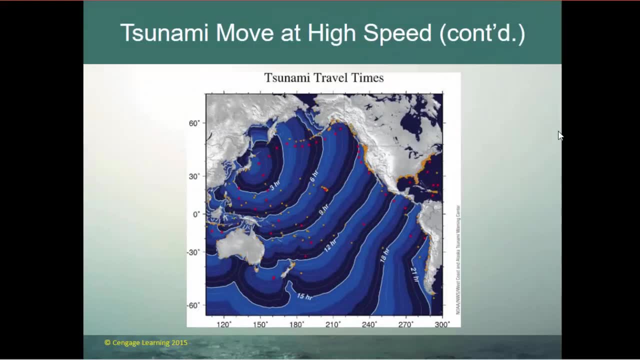 It took just under a day. So that wraps up chapter nine. Waves transmit energy, not water, So waves move energy across the ocean. Water does not move across the ocean surface, And the speed of ocean waves usually depends on their wavelength, And we showed you that formula back here. 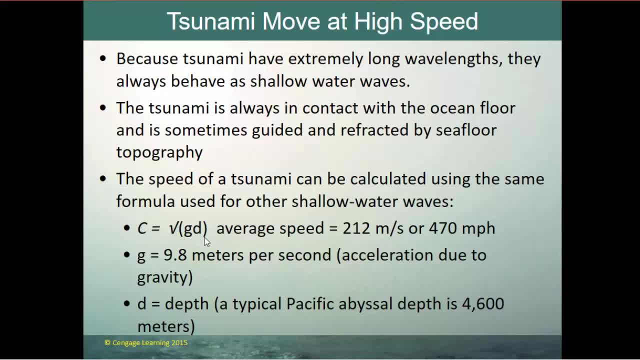 where the speed of the ocean wave is really a function of the depth of the ocean. The deeper the ocean, the faster the ocean waves, So as, because it's the square root of gravity, which is a fixed thing, 9.8 meters per second square. 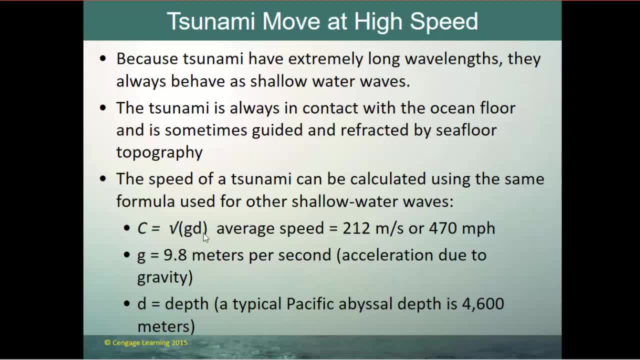 9,, yeah, .8 meters per second, times the depth. And so as the depth gets lower and lower and lower, shallower and shallower, the speed of the wave is going to get slower and slower. All right, the speed of ocean waves usually depends.